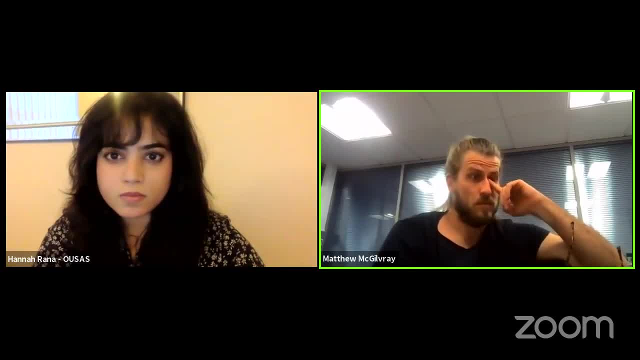 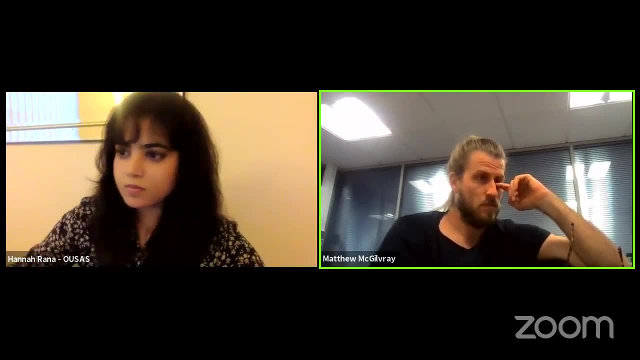 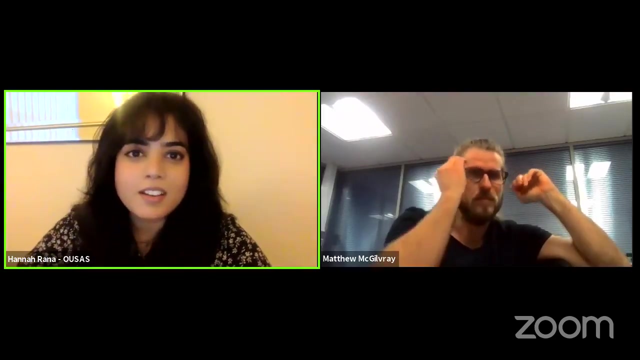 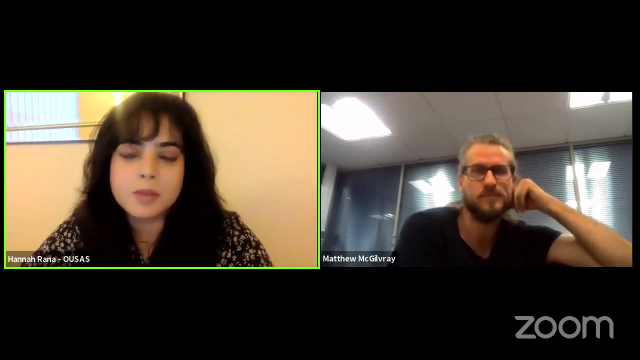 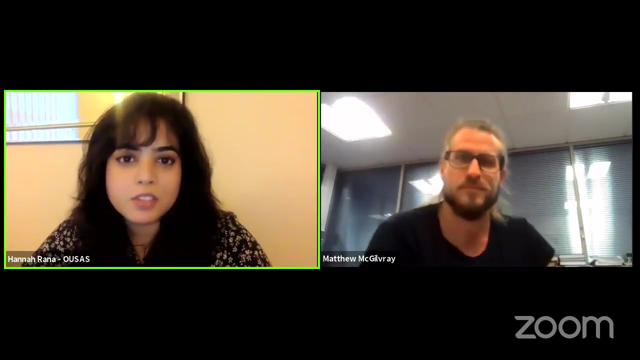 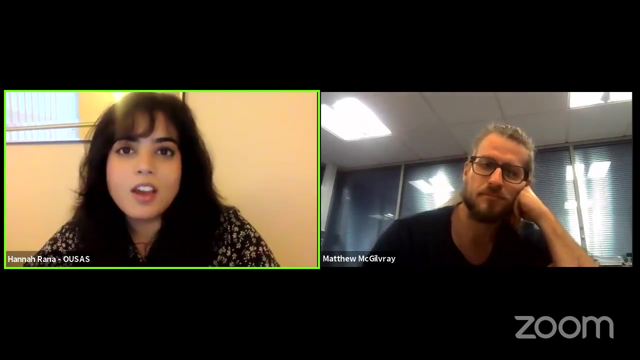 Okay, hi everyone and thank you for tuning in, the Oxford University Space and Astronomy Society is excited to be able to put on a few talks for you this Hillary term again entirely online and today we're delighted to have Professor Matthew McGillivray here with us to talk to us about hypersonic thermodynamics. So to introduce our speaker, Professor Matthew McGillivray is head of the hypersonics research group at the Oxford Thermofluids Institute. He received his Bachelor in Engineering and PhD from the University of Queensland. Over the years he has pioneered work in high-speed flow research and spacecraft aerothermodynamics and heat transfer and has developed the famous high-speed flow laboratory here at Oxford which involved the installation of the iconic high-density tunnel and the T6 talker tunnel which I'm sure we'll hear about more today. Professor I hear from your your DPhil students that you're incredibly busy right now with testing and so on so very very grateful to have you and to have your time. So without further delay over to you. 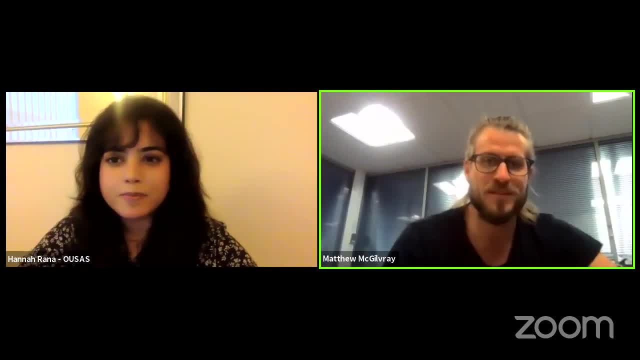 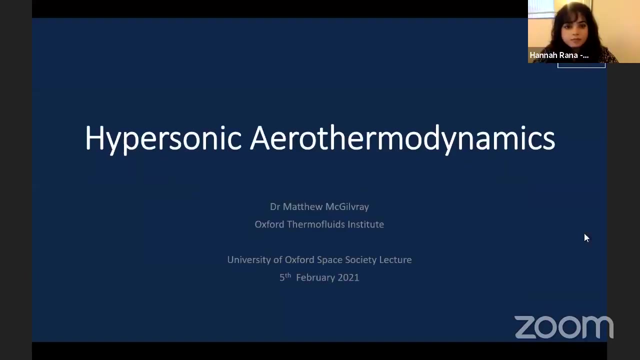 Thank you all for having me today. I'll try and share my screen here. You're able to see that yeah that's great. So today I'm going to really give a bit of an introduction to hypersonic aerothermodynamics and give you a bit of a first look at what we're going to be talking about today. I'm going to give you a few highlights of the research we do here in Oxford that many of the great DPhil students we have in the lab and fourth-year students in engineering have been involved in and hopefully you know if there's any questions are then very happy to answer anything from fundamental questions up to what we're up to here in the lab. So without further ado, so a bit of a background on hypersonic vehicles. 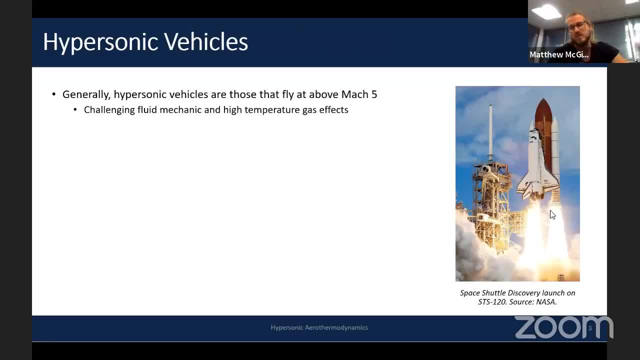 So, hypersonic vehicles are those that really are flying at incredibly high speed so five 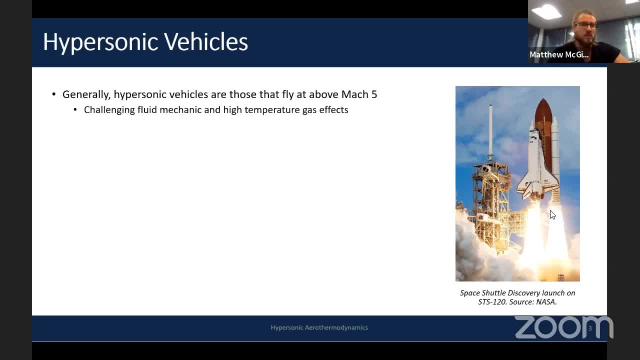 times the speed of sound so at sea level here we're talking nearly a mile per second and they create extremely challenging fluid mechanic and high temperature gas effects that we as engineers have to deal with when we're designing a vehicle that's got to fly. 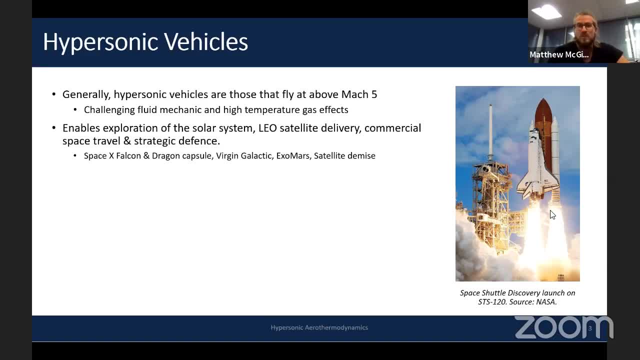 So, these things you know enable us to do a lot of things so from exploring our solar system to space travel to you know there's obvious defense implications of these and you're probably all very aware of all the different great systems that the US, our European colleagues within ESA have flown and there's lots of new players in the game. 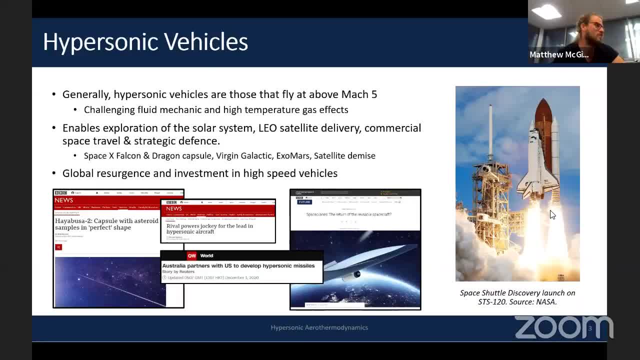 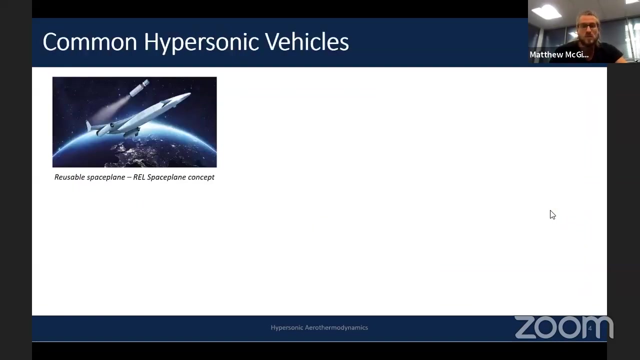 and this is really recently we've seen a huge resurgence in high-speed vehicles and really the underpinning investment and that's both from a civil point of view so you would might have seen recently that the Japanese flew back the Hayabusa 2 after capturing it to development of new opportunities with delivering payloads to low earth orbit or civilian transport at very high speeds all the way through to defense requirements and you know that's really being forced in the west by developments in both Russia and China so to give you a bit of a background on what common hypersonic vehicles there are so we've got reusable space planes so 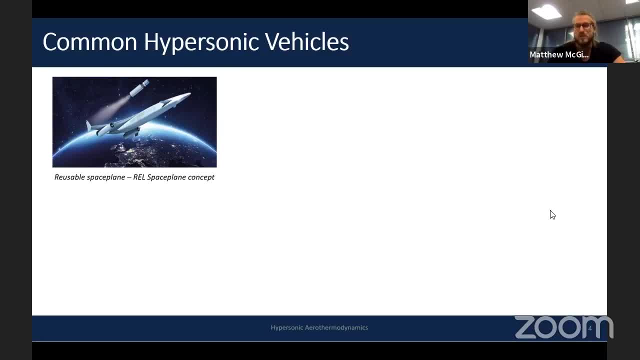 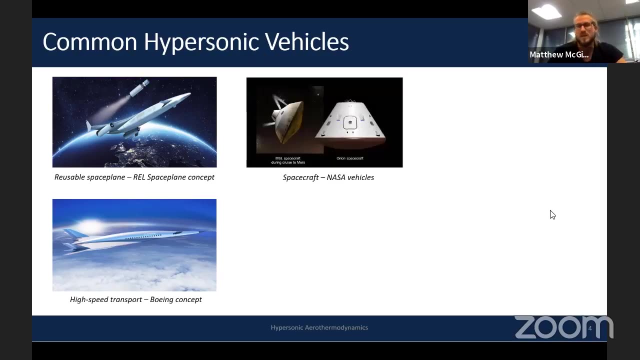 there are none of those at the moment there's quite a few concepts going around the space shuttle was one of them back before it was retired high-speed transport so we're talking you know really souped up Concorde here all the way through to spacecraft where we're going to enter at extremely high speeds into to not only earth's atmosphere but others 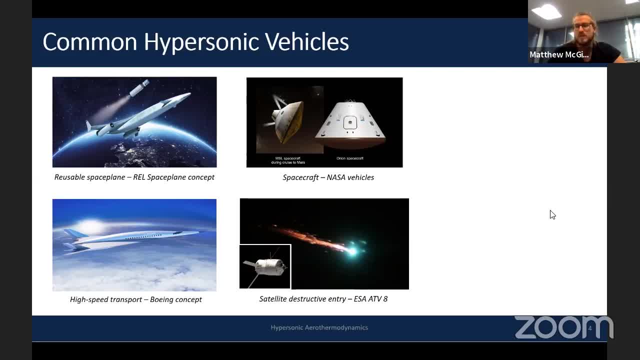 satellites so all these satellites that are up in space once they come to end of life there is now it by law you have to actually destructively enter them and so they'll come back at you know 30 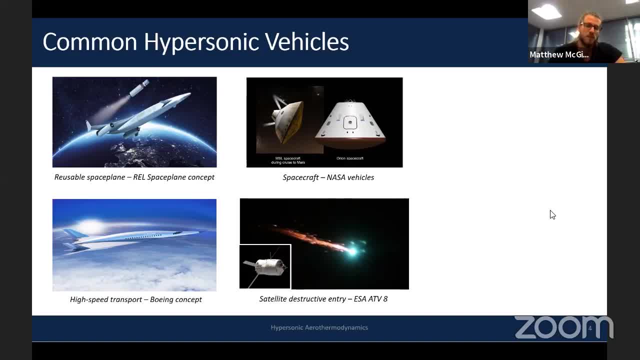 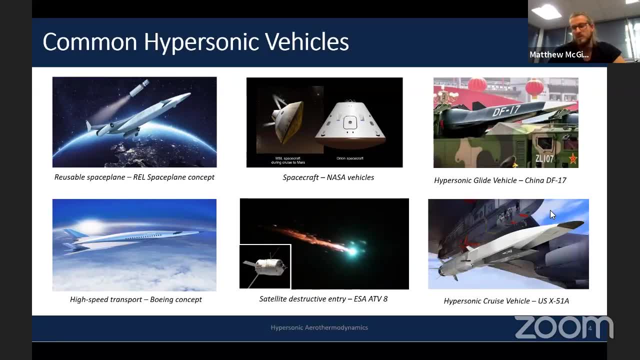 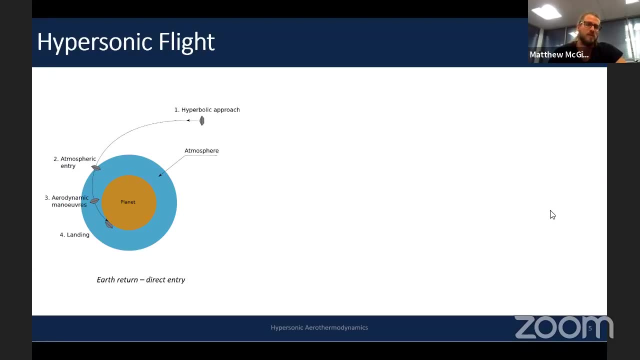 times the speed of sound and but all the way through to defense systems like hypersonic glide vehicles and hypersonic cruise vehicles so if we're going to come back to earth we're going to come back on a very very fast 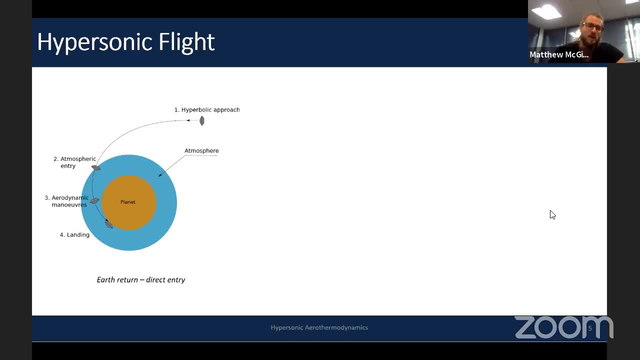 spacecraft and we're going to enter the upper atmosphere and as we as we hit the atmosphere we can then start producing aerodynamic lift and aerodynamic drag but whilst we're doing that we want to keep stable but also we have to manage that there's going to be extremely high heat fluxes when we do that so if we look at a trajectory plot of the sort of speeds and 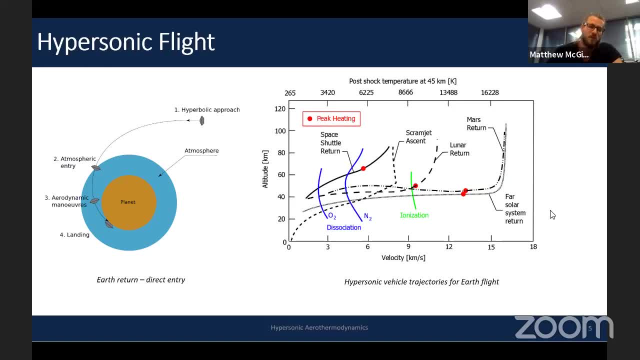 altitudes we're interested in for earth trajectories you know over at the kind of more moderate speeds uh what it's going to take us to get up into space 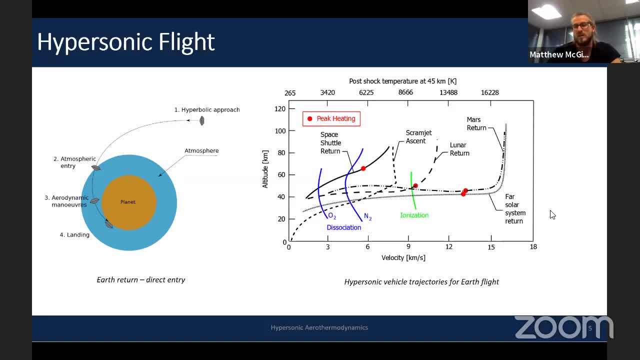 but when we start moving out towards the right in terms of the entry speed from high altitude you can see it starts off with a space shuttle from low earth orbit but then you're moving out to 10 k's a second for lunar return missions and all the way up to 15 16 kilometers for mars return and fast solar system return so the speeds are always increasing but if we want to go to jupiter then we're talking stupid crazy speeds of 50 kilometers a second 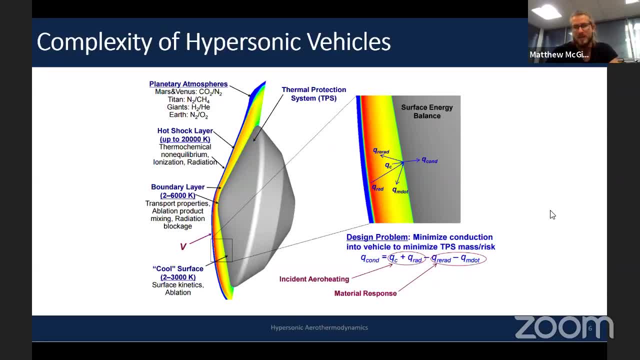 so without going too deep into this slide it's really here just to say these things are complex um we're going to be producing all kinds of high temperature gas effects from you know lots of chemical reactions to to generating non-equilibrium energy states within our gas and the gas will start ionizing and radiating all over the place if we want to go to different planets we've got to deal with very very different gases that we're flying in down at the vehicle itself we've got a series of complex processes going on especially when you start having an ablative heat shield 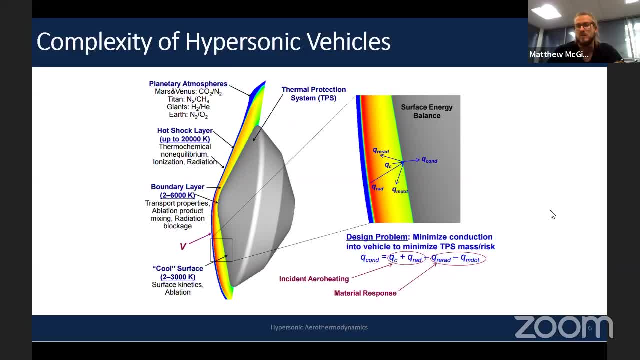 and all those things need to be thought about if we're going to make make a heat shield that will actually fly 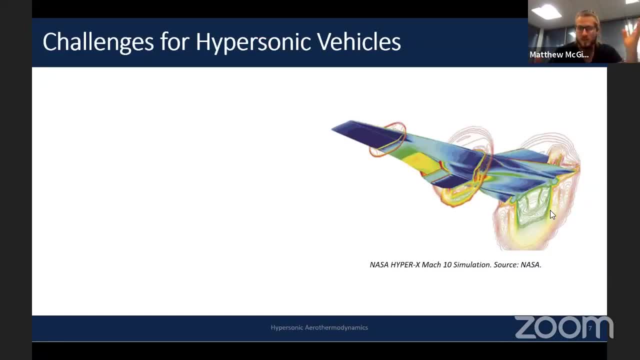 so to give you a bit of an overview of i guess where the challenges are for us engineers in the room that want to go build a hypersonic vehicle full time time's an obvious one if you're flying over 4 000 miles per hour you know any perturbation any change you've got to be fast at reacting and there's just not much time to to do any changes so that's why we see a lot of very blunt vehicles that are extremely stable coming into earth's atmosphere so if we want to fly over that huge trajectory range where you've got you know you're running 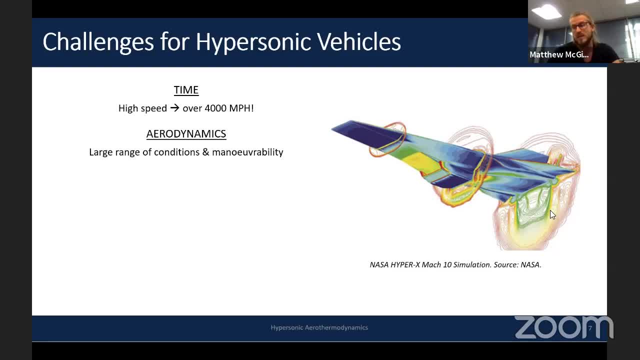 into only a few molecules of gas all the way down to sea level you've got a large range of dynamic pressures and you've got to worry about you know the structural loading to this vehicle dynamic stability if you start maneuvering it's extremely difficult heating so you know we're going to have air hotter than the surface temperature of the sun it's going to generate a lot of heat transfer to the vehicle thermochemistry so i've already mentioned that there's just complex coupling of physical processes and the chemical species that are there and finally we just don't have to really perform high-fidelity numerical simulations for these vehicles. 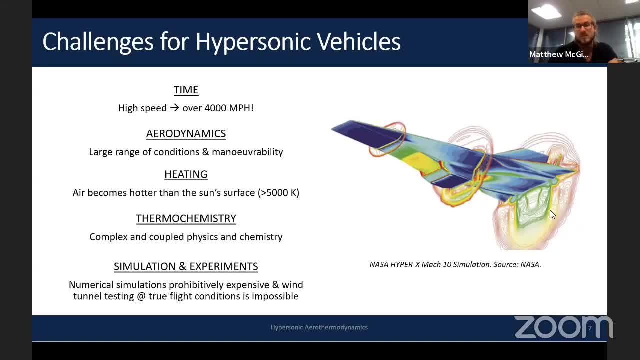 And wind tunnel testing at actual flight conditions is just impossible. 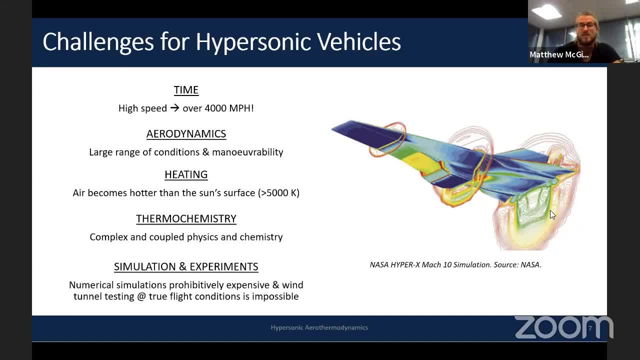 So essentially, the first time a lot of these things get tested is actually the first flight test. 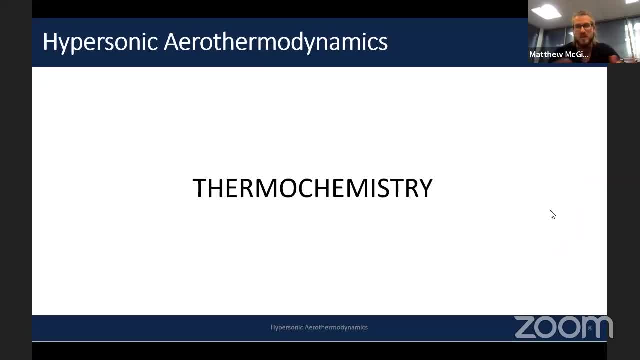 So I'm going to touch on a few of those points because I don't want to keep you here all night. So we'll start off with a bit of thermochemistry. 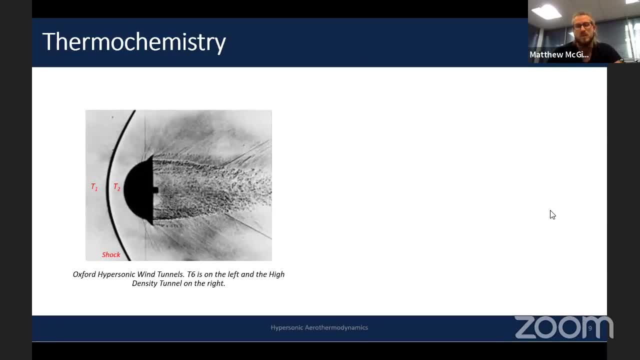 So if we think about a high-speed vehicle, it's going to generate a shock in front of it. 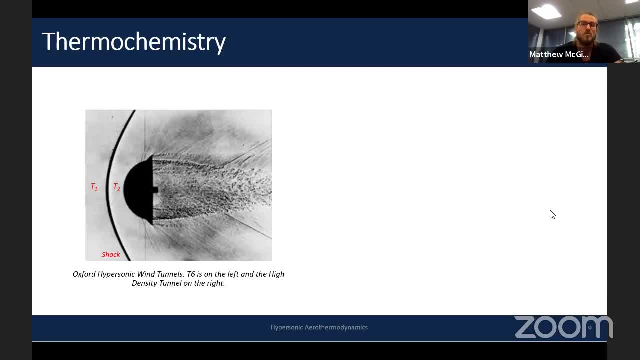 So a shock is generated when you really need to compress the flow to move it out of the way. 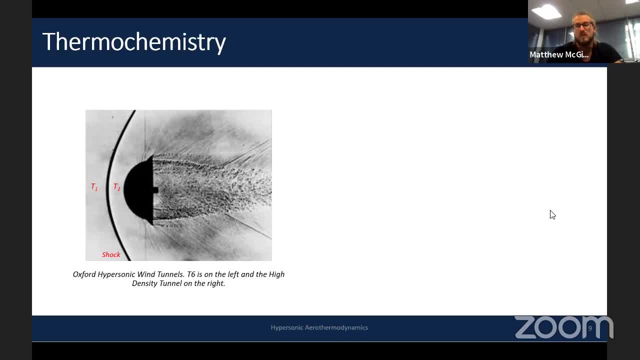 So in the shock's frame of reference here, the gas would be coming left to right rather than the vehicle's frame of reference where it's flying towards the left. 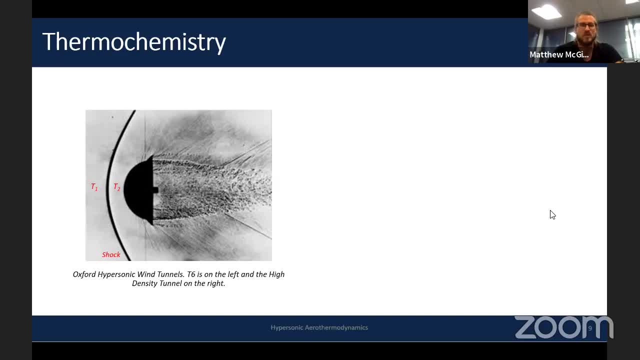 And as the gas passes across the shock, it's going to become very, very hot. And if we treated that as an ideal gas, which you might have studied in some of your earlier years, we'd be getting for entrance speeds of six kilometers a second, we'd be getting up to 20,000 Kelvin. 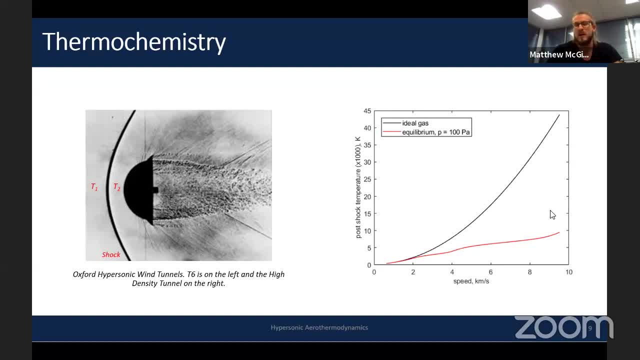 But that doesn't really happen because we start getting chemical reactions occurring and it comes down to we store some of that energy by dissociating some of that energy from the vehicle. 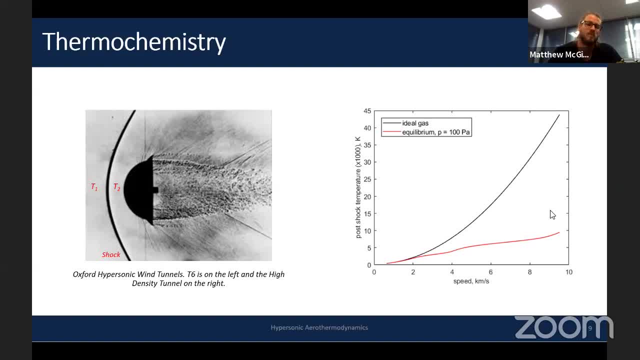 So we actually get a decrease in the temperature back down to a lovely moderate, you know, 6,000 Kelvin. 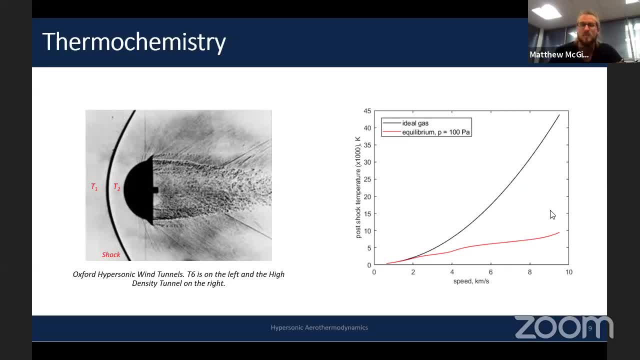 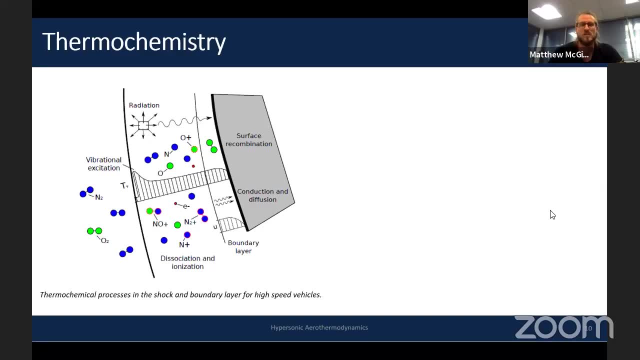 And so, you know, that's equilibrium thermochemistry, but it's actually quite a bit harder when you start going higher and higher in speed, you need to worry about lots of more coupled effects which are going on. So if we look at our oxygen and nitrogen, we're going to see a lot more of that. So if we look at our oxygen and nitrogen, we're going to see a lot more of that. So if we look at our oxygen and nitrogen molecules, 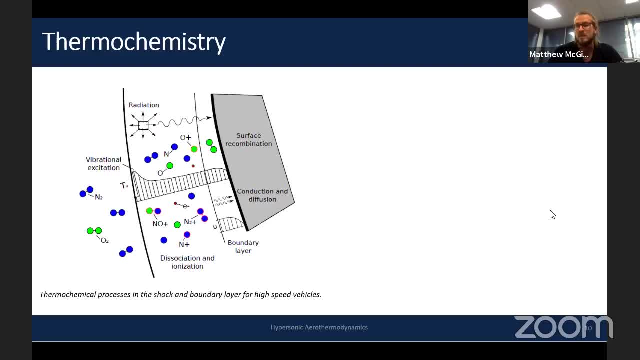 as they pass across that shock, they might become dissociated. 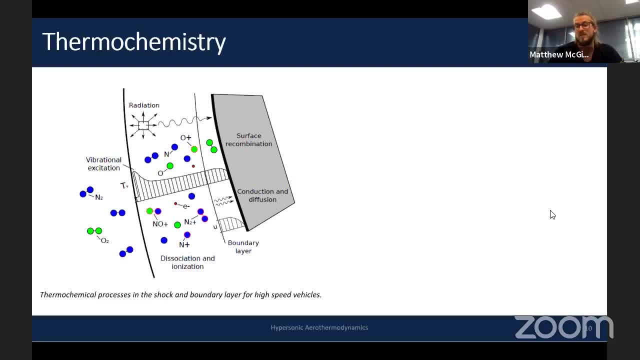 They might get energized into higher states. So particularly vibrational excitation. 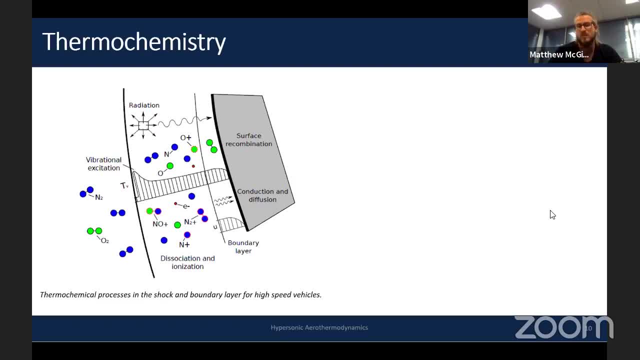 And that will then take a certain resonance time for both those energy states to come back down to an equilibrium level with each other, but also for all the chemical reactions that might occur. So, you know, generation of NO plus there. And if we're going fast enough, we might even get ionization, so we'll have lots of free electrons. And if that gas gets hot enough, particularly in that non-equilibrium region, we'll then start getting a hell of a lot of radiation from the gas itself towards the vehicles. 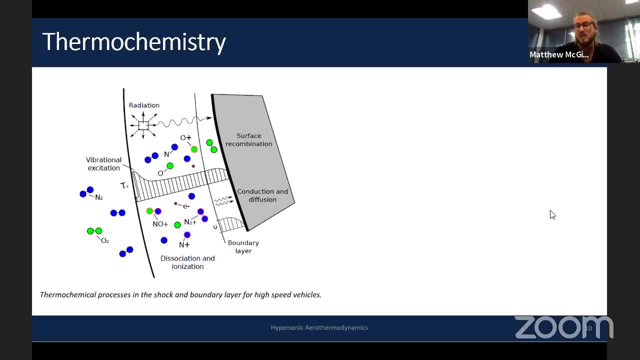 So once you're over 10 kilometers a second, coming back to earth, the radiation dominates the amount of heat flux you're getting to the vehicle. 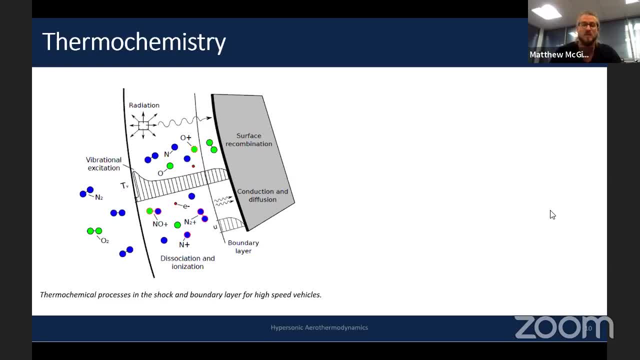 So it's actually just dominated by that hot plasma front of the vehicle. And as we move up in temperature, we're also generating those different species, so we'll actually get radiation in different parts of the spectrum. And some of that might be absorbed by the gas in front of it before it reaches our vehicle, but it just depends 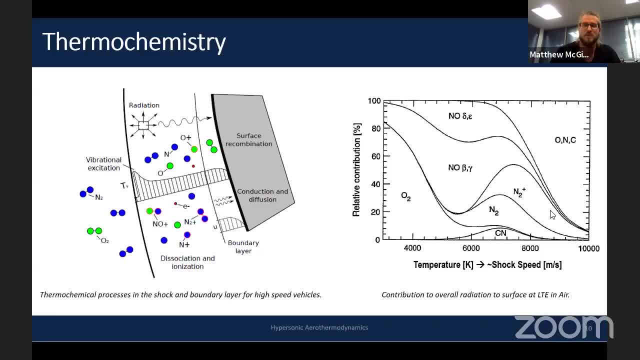 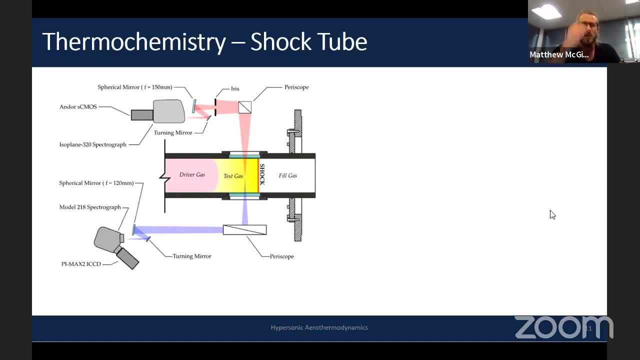 on what's present and what's BBR and in what quantity. So how we study it here in Oxford is to perform shock tube experiments. So some of our great students here have set up an experiment where they pass a shock down through an ambient test gas. So you can imagine instead of what's 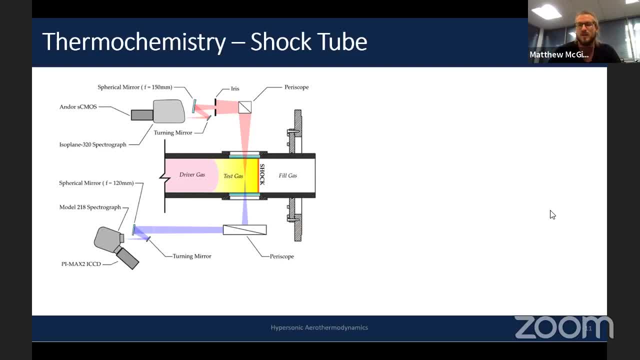 described there as a driver gas, it's analogous to us firing a spacecraft down our tunnel. So we set it up just like it would be for a flight test. So our fuel gas could be air, if we're simulating earth entry, but it could be a mixture of carbon dioxide and carbon dioxide. So we're going to first test the gas to see how much carbon dioxide and nitrogen, if we were simulating a martian 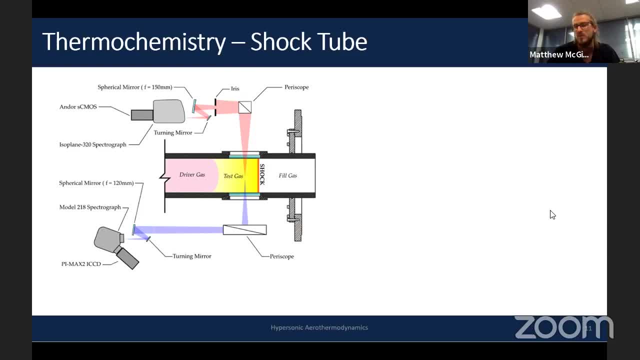 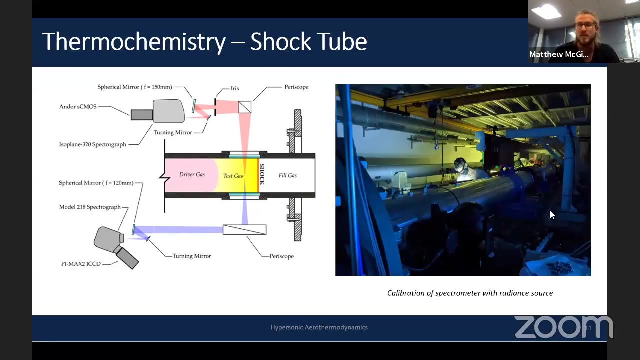 entry condition. And the shock speed is really equivalent to our entry speed of our vehicle. And so we capture some of the emission of that radiation that's coming from that hot plasma behind the shock. And we pass it on to two spectrographs, which break the light up into wavelength. And then we image it on some cameras. And if we perform some pre-calibrations of of those cameras and the wavelength spectra we can then actually start getting quantitative data out of these things. So just to show you what a test looks like. 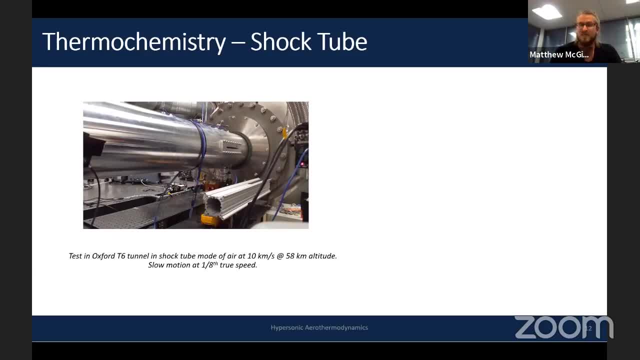 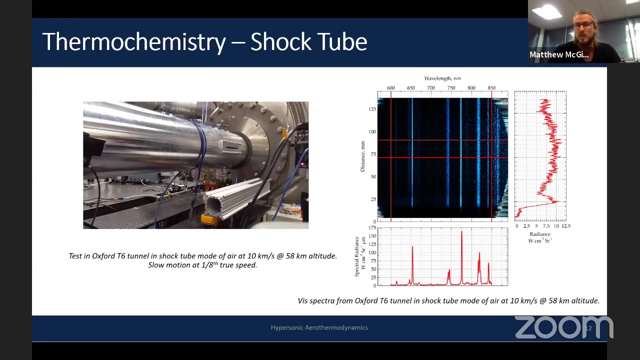 A bit of slow-mo there. So we don't even just have we don't have a long time to capture it. So it takes us about between four to six hours to set up an experiment and we get about 20 nanoseconds of data to 200 nanoseconds of data. So a lot of brute force to get a very small amount of data but this data is extremely valuable currently where there's only us and NASA that are capable of performing these experiments at the moment. So and there's nuances in the NASA experimental setup that they're actually very keen on us forming these because they think there's big uncertainty. 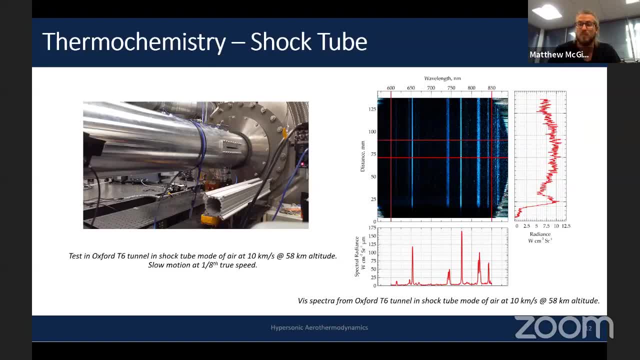 And you can imagine if you if you put a bit more radiation into the system or you have different thermochemistry your aerodynamics could be off or you might be getting a much bigger heat shield than you want to. So or you might be burning up in the upper atmosphere. 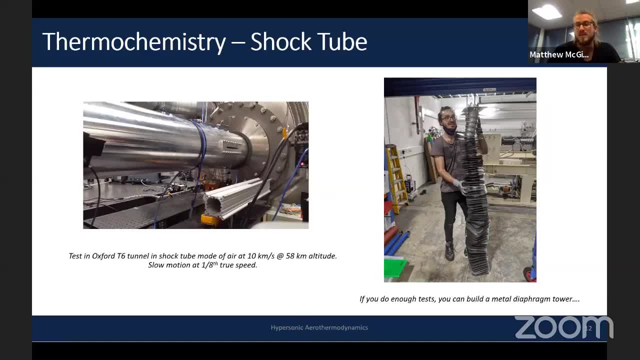 None of those are good. And if you do enough tests you can build yourself a metal diaphragm stack even taller than yourself but that's what you get after being a PhD student for four years. 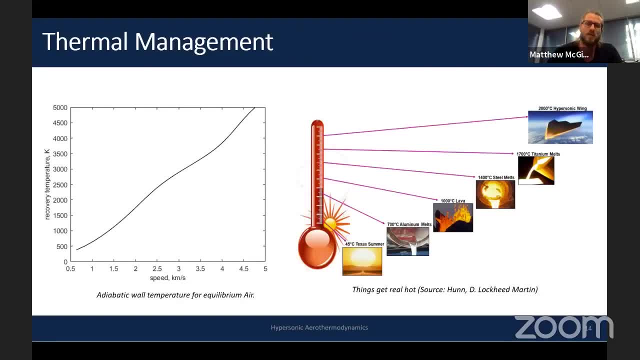 Thermal management. So if we think about what the possible temperature of our material could be it's really it's nearly the post-shock temperature. There's a there's a small deviation from that but so and it it works out it's about linear you know five kilometers a second is about 5000 Kelvin. 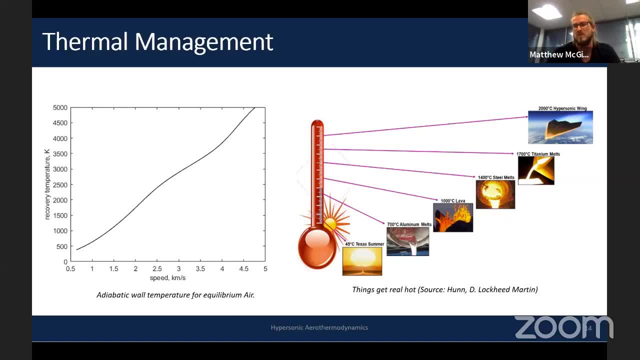 So it's a really big difference in the amount of possible temperature that you could get to at the surface if you actually reach equilibrium. But we obviously have some cooling mechanisms involved. 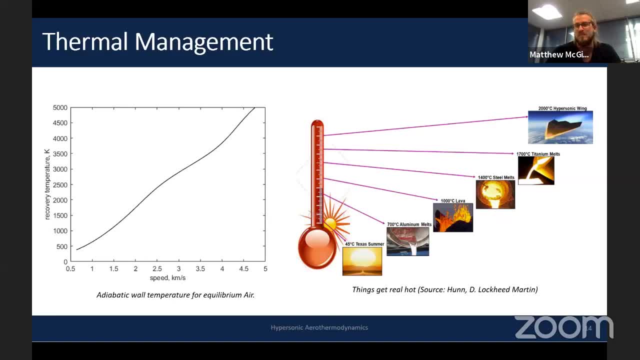 But just to think about what what different temperatures mean you know we're starting to 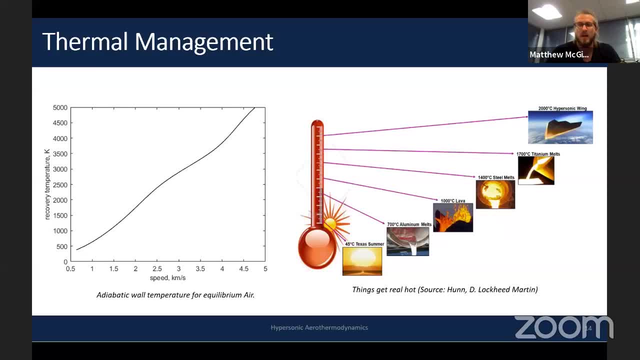 melt all metals above you know 1600 Kelvin. Up above 2000 Kelvin you definitely melted all metals. 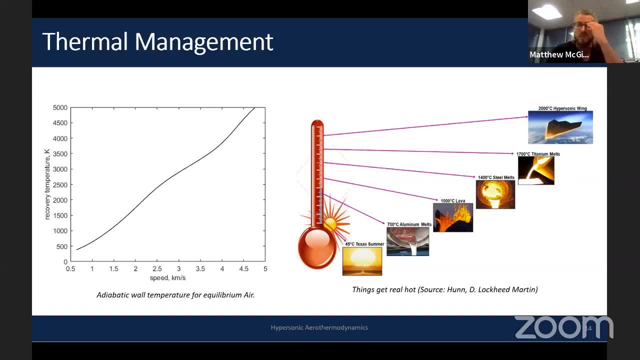 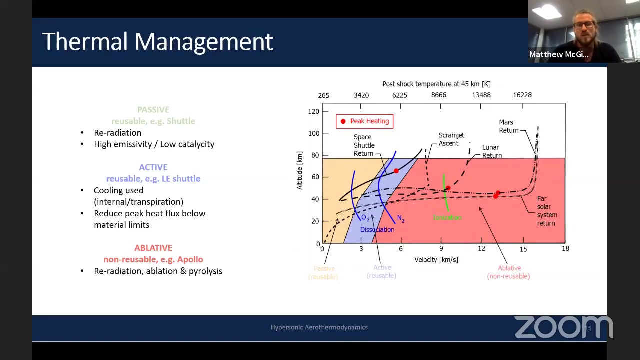 But if we want to be flying you know at two three kilometers a second so we want to jump on a a nice space plane and and ride around or if you've got a defense application and you want to have high high aerodynamic efficiency you're going to need to get your leading edges of your vehicle much above that melting point of the material. So there's various choices for us when it comes to cooling technologies. And the best being passive because they're robust they'll work every time but they're limited to to lower speeds because once you get high enough as you just saw all of these materials start melting away. So then we can start thinking about active cooling so where we might have a heat exchanger inside the the wing itself or we can have a transpirant that passes through the material and out onto the outside. 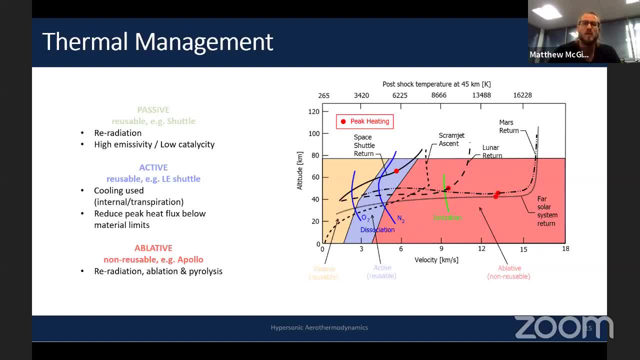 Creating a cool blanket around it but that that allows reusability but again once you go high enough in temperature again that won't survive. So we we then need ablatives and ablatives are very good because they're they're low complexity but they're always shape changing. So you've always got a different shape of your vehicle and they're just extremely difficult to model. 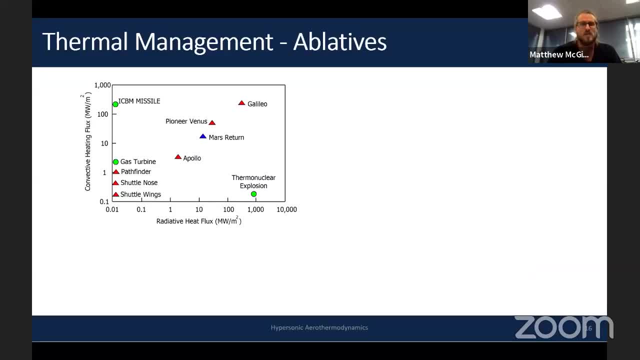 Which hopefully you'll see in a few slides time. So if we think about some of the numbers involved that they're absolutely bonkers crazy. So you know the shuttle was just getting a moderate 0.1 to 1 megawatts per meter squared and that's kind of able to be dealt with you know you can remember the the tiles on the space shuttle and a big kind of carbon bit on the front. And you know you can 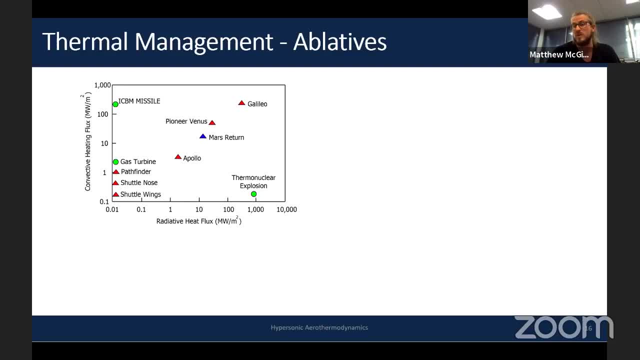 see your modern gas turbine can you know handle those temperatures just by by using film cooling. 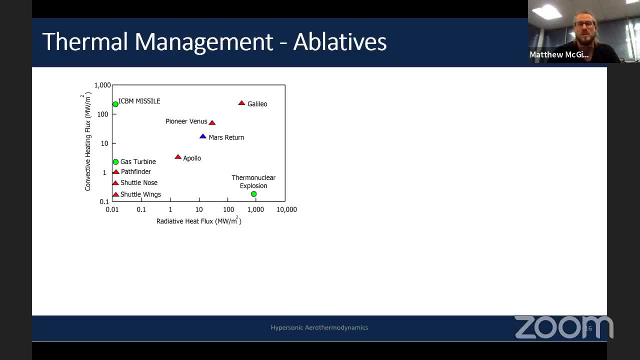 But if we start looking across when when we hit Apollo which was entering at 10 kilometers a second 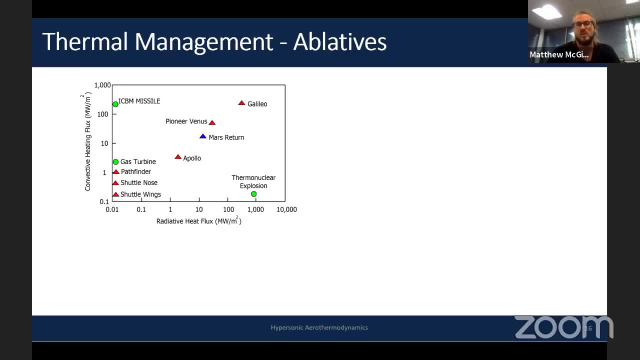 you know radiative starts taking over and you get a huge increase in the amount of radiative heat flux. And so by the time you're entering Jupiter at 50 k's a second you know you're taking on the convective heating that's seen by an ICBM missile. You know you're taking on the convective heating that's seen by an ICBM missile. 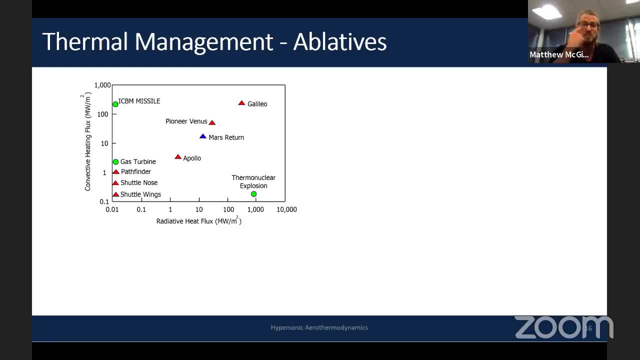 And a thermonuclear explosion you know you've got to design a system to survive both of those things at once. And it's not just about the heat flux into to the surface it's also about the integrated heat flux. Because if you're using an ablator the longer you fly out of that heat flux the more ablation you're going to have and therefore the more thickness of heat shield you're going to need. So it just so turns out that as you increase that total heat load essentially you're minimizing the the mass fraction you can use for your actual payload. So really as engineers we're thinking about how can we minimize that TPS mass fraction. And there's a lot of work that's needed to be done. So we do work here like I just showed with the thermochemistry and shock tube experiments. Where we're trying to measure the radiation a lot more accurately. So you can reduce the margins on that. 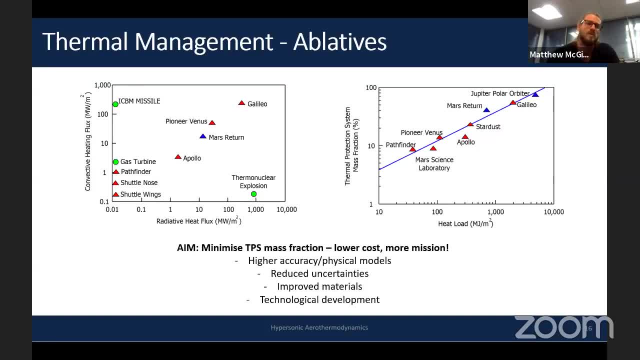 um but it could also be to to to think about how do we um get a get higher a better knowledge on 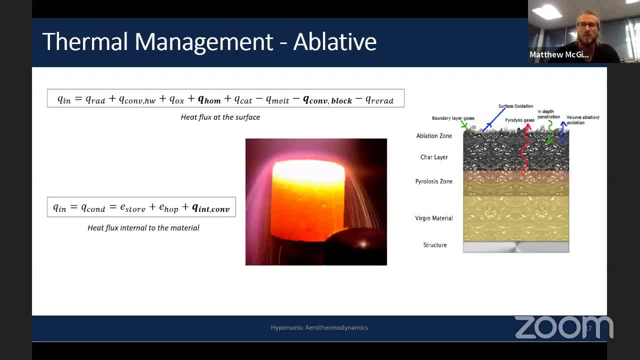 what that can convective heat flux is and one of the big um difficulties with ablators in themselves 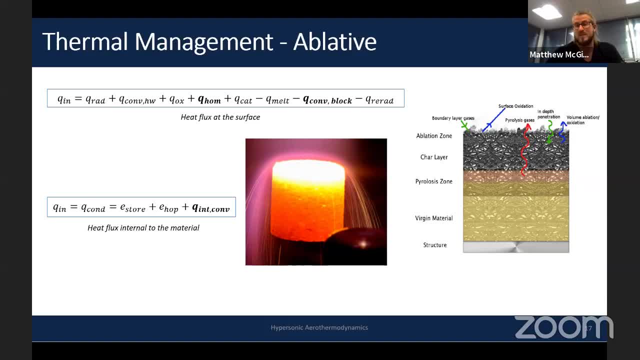 is that just the pure complexity of all the processes going on at once so i thought i'd put two equations in this presentation um sorry about that um but it's more just to highlight 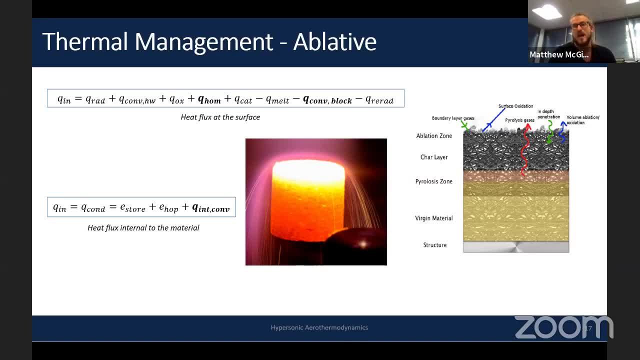 all the different things going on so the top equation is saying how much is the heat flux into the surface of the ablator so you've got radiation from the gas coming in you've got 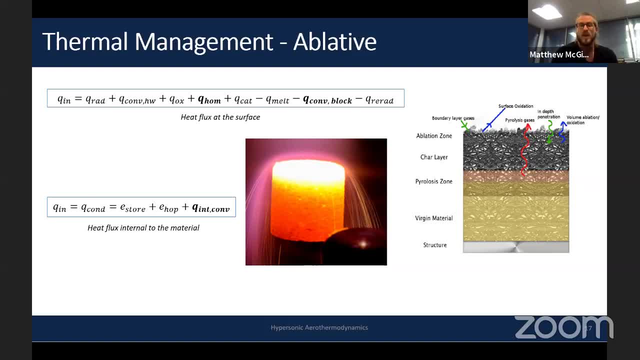 convective heat flux due to to the hot gas passing over the top of it you can have an oxidation heat flux because you're starting to to pyrolysis your um tps and that um epoxy resin is starting to come out you can actually get combustion of it 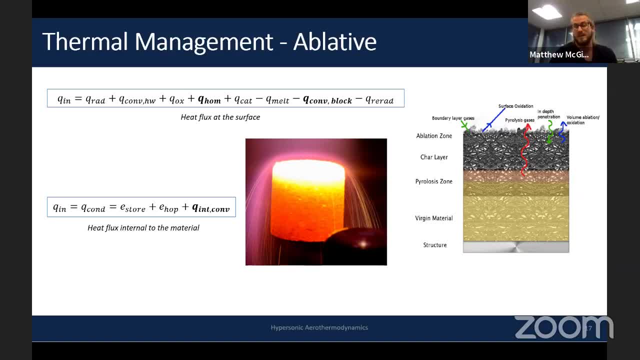 which then adds an additional heat flux in you can have catalytic recombination of your um 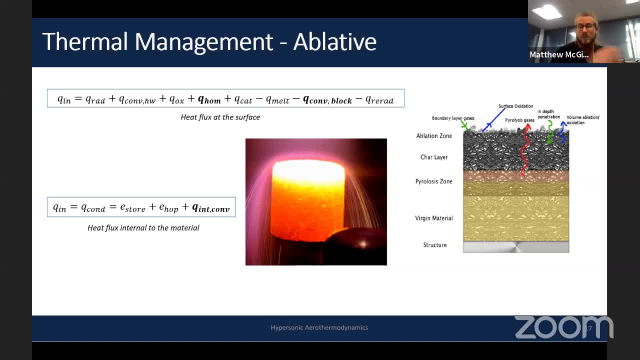 of all these species which you've you know heated up to incredible temperatures and dissociated um then you've got some bits that reduce so we could melt so that's going to 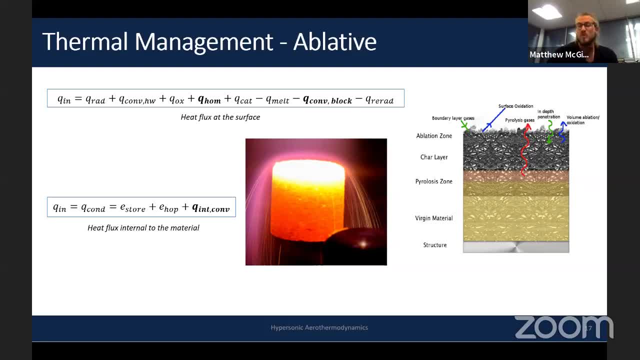 absorb a bit of energy we can um because we're passing blowing a gas out on the surface that's kind of like a gas turbine's film cooling system and because this material is getting really really hot it can re-radiate back out so we can get somewhere and similarly the heat flux actually 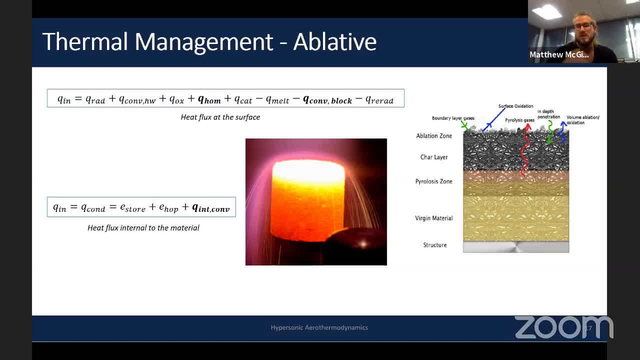 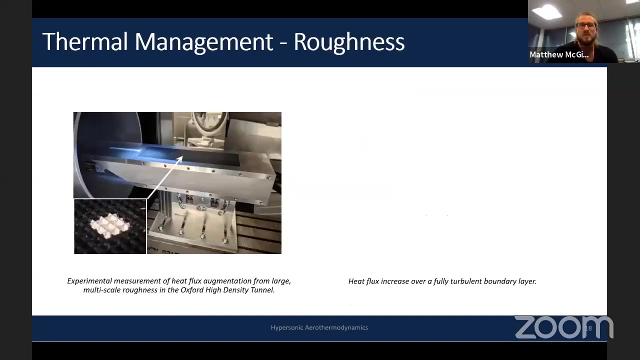 going in we've really got you know it's the conduction going into the surface can really only be going to three places right so and the being in the surface is going to be a bit colder than the um the the leftover fibers which is passing through but ultimately these things are just you know it it blows my mind every time i see these they're just super complex and we're still modeling them with very simple empirical correlations which just wash over all of these physical processes and we tune them to to one of the most important things that we're going to be able to do in the future so we're going to be able to do a lot more things with these things so we have a lot of work to do with these things but we've also put together one set of experiments at the end um so we kind of fly blind with these things so one of those things that we're working on in the lab here is to think about um what happens to that char layer and the convective heat flux which is one of the biggest contributors and so essentially we're built to model we put in our high density tunnel here and we've built 3d roughness patterns where we have different gauges which will have um measure the that heat flux so we do it in three ways we can do it either a with a silver calorimeter gauge 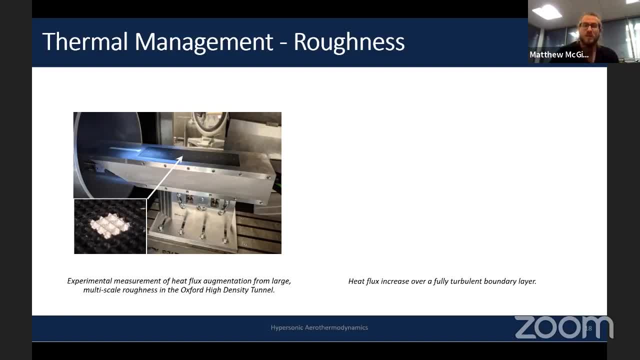 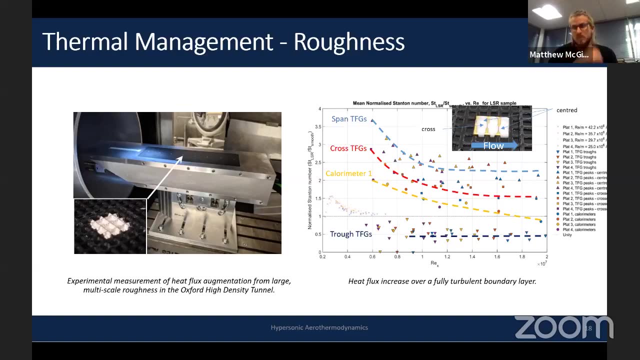 where we measure the temperature of a lot lumped mass and we can then infer back what the heat flux was we measure the surface temperature with an ir camera and again have a way of back processing to the heat flux and the final is thin film gauges which are just essentially resistors which change their resistance depending on temperature and so we can back out again heat flux from those 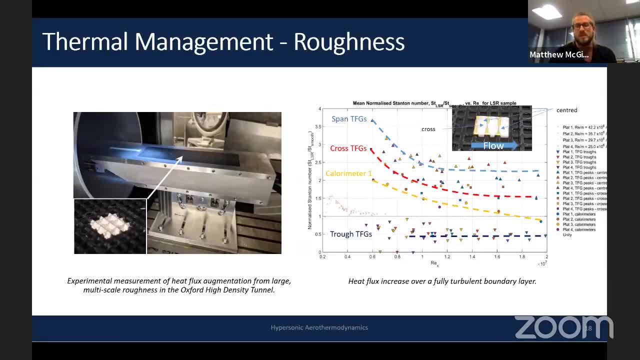 and you can see the these are really heat flux augmentation numbers so as we move down that rough plate you can see we're getting incredibly high heat fluxes particularly on the tips of these things so that's where you start getting shearing because these heat fluxes are so incredibly high the material becomes very weak even though it might be a carbon fiber 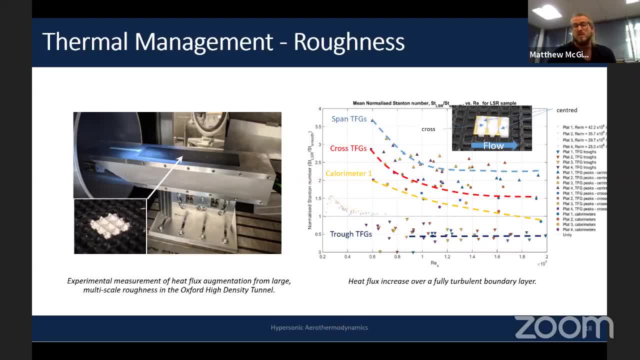 and start start getting sheared away so that that's really the motivation that you're getting very very high heat fluxes on the top and above what we just predict from a simple turbulent boundary layer at the top because it's so rough these these roughnesses tend to be 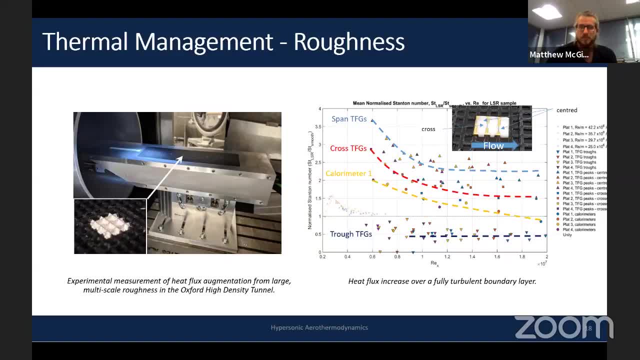 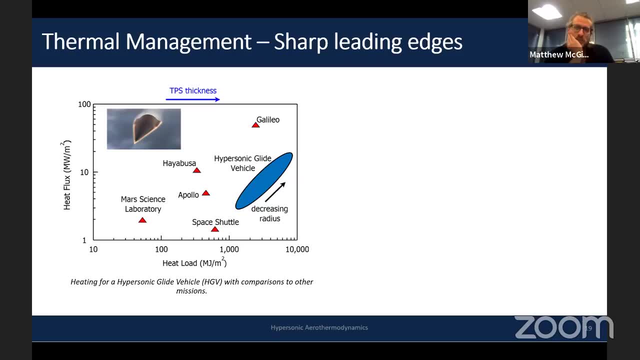 on order of the size of the boundary layer um so that's good for for space vehicles but what if you're interested in flying a more aerodynamic 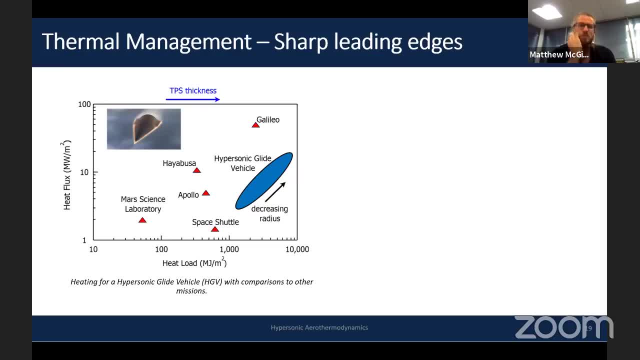 um vehicle so a glide vehicle or um maybe a space plane um so i've plotted taken those two axes we 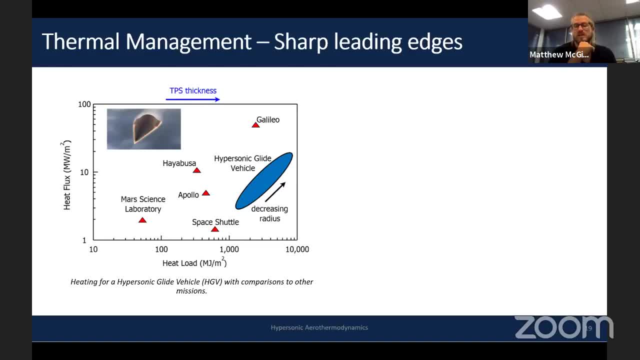 saw a little bit earlier of heat load and heat flux and then re-plotted all of those different emissions and so what you're seeing is when i put in that big blue bubble for the hypersonic glide vehicle that although the heat flux is 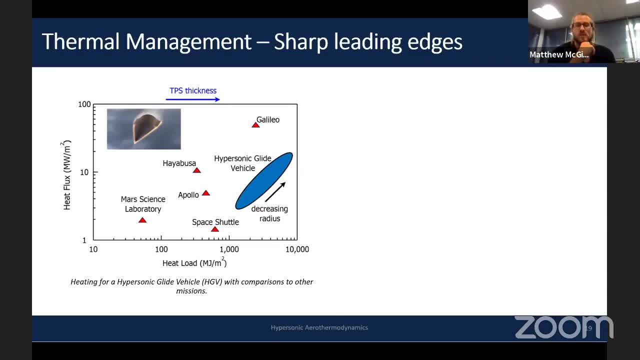 kind of things we've flown before in earth's atmosphere so the apollo emissions high abusa the heat load is nothing like what we've done before and if you want to get to to higher aerodynamic efficiencies you need smaller radiuses and that's just going to drive it higher to higher heat fluxes and higher heat loads so it it's how do we deal with this so one potential avenue would be to to go to a really super duper 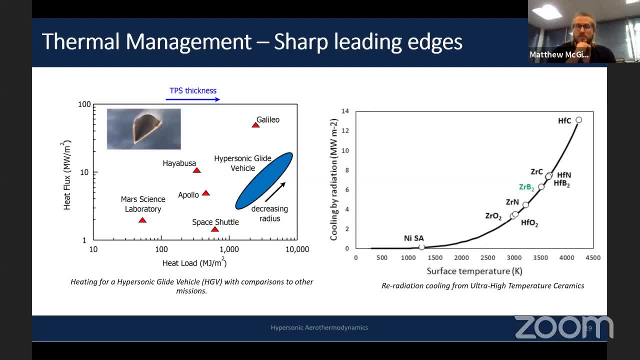 material in the future like ultra high temperature ceramics and they they they have some promise so you know we can get up to really high temperatures so we're seeing with hafnium carbide there 4500 kelvin because we can re-radiate out lots and lots of um energy which will therefore do our cooling um so that's that's fab we might be able to just get away with a passive system but if we're able to do that we might be able to get away with a passive system um so that's that's fab we might be able to just get away with a passive system with these new new fancy materials um the only issue is that these things don't work above about 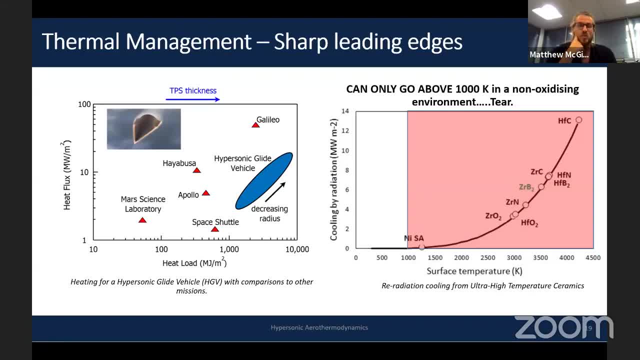 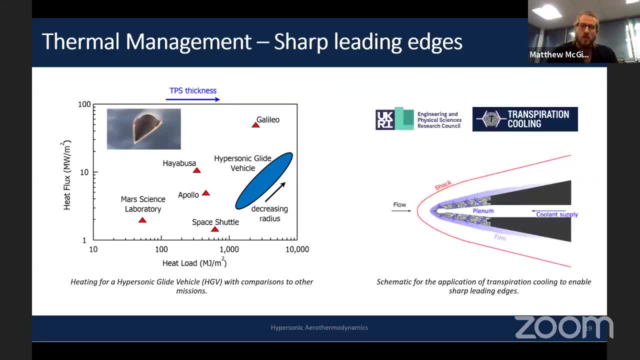 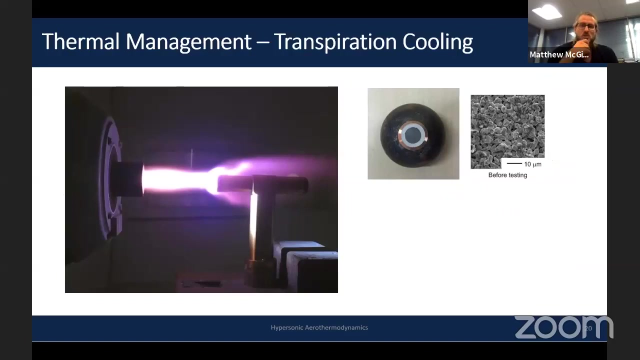 a thousand kelvin in air because they just get destroyed by oxidation um so that becomes a bit of an issue so um we've been doing some work here over the last five years um thinking about whether we can pass uh an inert gas out through a porous part of this ultra high temperature ceramic and create a little buffer layer between it and the oxides which are existing in our shock layer and protect protect our our leading edge so it can actually just then re-radiate out um and to show you some of the tests that one of our students performed over in stuttgart in a plasma wind tunnel so um the plasma wind tunnel test is shown on the left um you can see the probe head which would have been facing the the floor flow there and in the middle you can see some ultra high temperature ceramic that's actually porous so the close-up microscope image is on the right and you can see it's made up of little spheres that are fused together and you can see it's kind of porous so if we don't do any cooling it oxidizes and gets destroyed very quickly it doesn't survive very long at all but if we start passing some nitrogen through it it survives completely so it proves the point that we can actually block any of these oxides getting to the surface by creating a gas layer but what we pay for over a passive system is higher complexity in in in the engineering 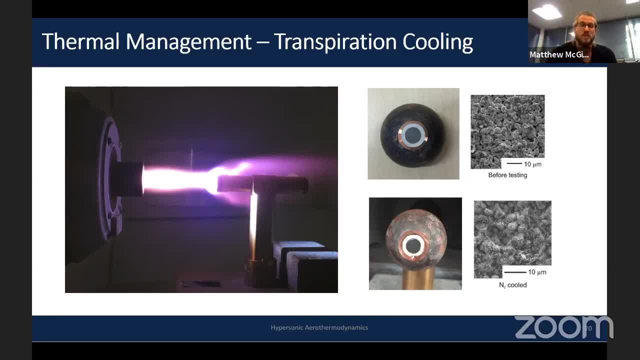 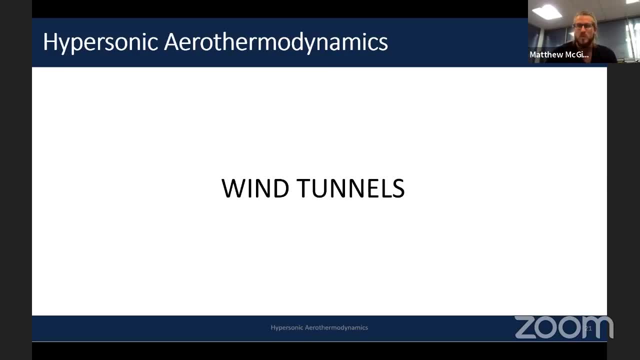 solution so there's more risk of failure of this thing okay um i've got about 10 to 15 left so i'll try and get through just a bit of what we do here with wind tunnels 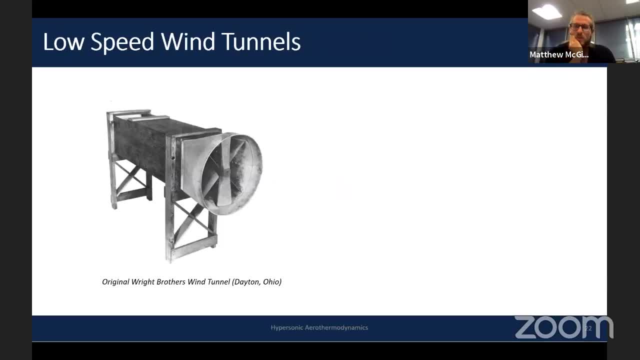 so um most people might have seen or um at least you know heard of a wind tunnel before so the original creators of this were were the wright brothers to to start thinking about um you know their their airfoil shapes for for wings on planes and so um essentially it was just a little fan with um a nice little square test section where they could put in different airfoils and measure pressure 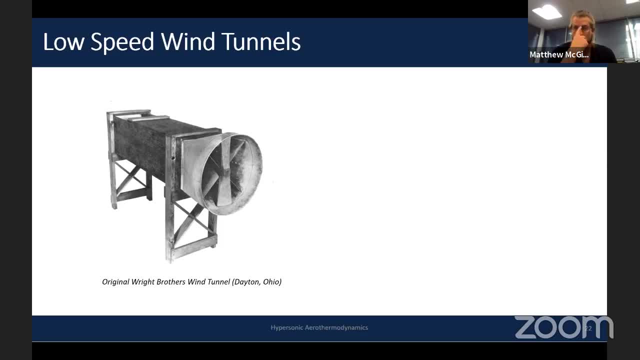 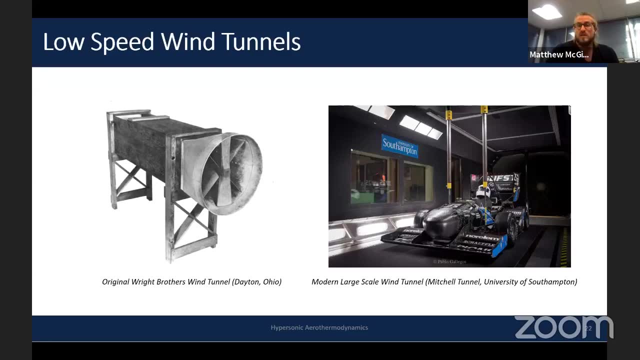 lift coefficients and drag coefficients on these aerofoils and you know essentially for low speed wind tunnels the modern modern wind tunnel is essentially just a super scaled version of it essentially they've got much bigger fans and much bigger test sections to the point where they can even fit in whole you know or scaled versions of formula one cars and they've got lots more measurements that might take laser diagnostics but essentially that that stayed the same 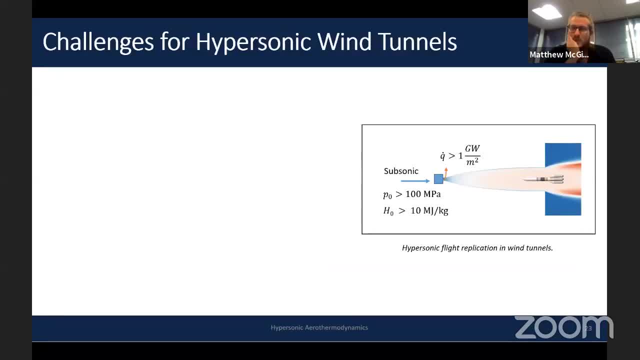 but hypersonic wind tunnels are a bit more challenging we can't quite make them out of timber and perspex so if you wanted to drive a hypersonic flow essentially you normally start from a stagnation region where you where you're going to have hundreds of hundreds to thousands of 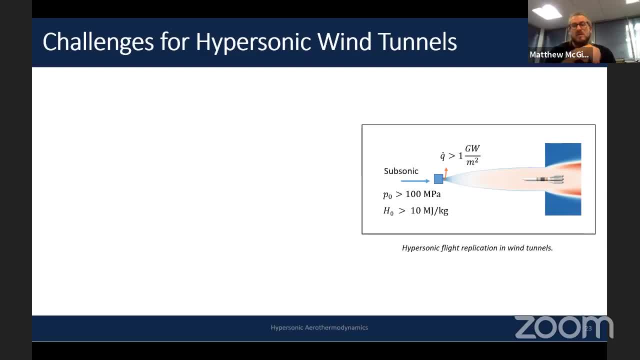 bar of pressure and really really high temperatures and that flow is then going to pass through a converging diverging nozzle and then over to onto a scaled model and the difficulties come that you know if we want to get to a to decent model sizes or to replicate our non-dimensional quantities that we want to like reynolds number you're going to have to to to have a nuclear power plant sat next to you to to drive the thing um you know the pressures are high and you've got to contain them in that stagnation region so it's you know you bottom of the sea sort of levels of pressures um the heating is like an order of magnitude higher than on the space shuttle um main engine throats which were completely ablative and replaceable um we've got to deal with these things in in testing um so we have to match the gas composition that's natural in the atmosphere and if you start with a really really hot gas in that stagnation region and then pass it expanded back out it might not have enough time to to come back to to a nice you know oxygen nitrogen mixture more likely you've got a lot of not um no sat in your flow which means you're not matching the gas composition or if you use a vitiated heated facility where you're burning fuel and burning 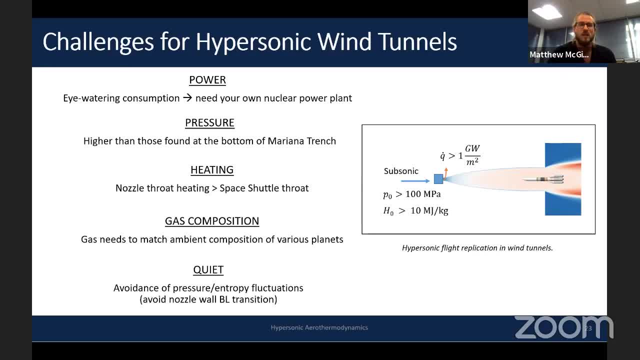 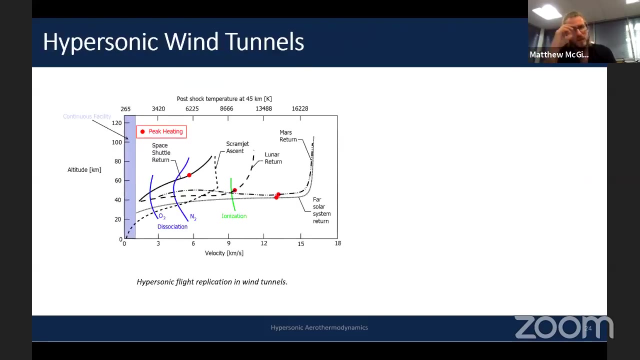 oxygen you're definitely not matching it and and ultimately if you're interested in boundary layer transition experiments whatever drives the processes from the left there can't be causing huge fluctuations and you can't have a transition of your boundary layer on the nozzle walls radiating in a bunch of noise so we've got to think about it a bit further so to have a look at what sort of hypersonic wind tunnels there are bringing us back to that same plot of trajectory um if we want to have a continuous wind tunnels that they're essentially pretty cold and very low speed in comparison um so but there is one exception and that's plasma wind tunnels which can run continuously but they don't match any of the other aerodynamic quantities so they're good for the materials testing but they're not very good for any of the aerodynamics or radiation or convective heat flux problems um so if we look at blowdown tunnels there's there's various different types um there's ones where you store a lot of hot air or pass them through heaters on the fly um and then you pass it through that converging diverging nozzle into a big vacuum tank at the end so high pressure wants to go to towards low pressure and they they they allow us to get run times of seconds to hundreds of seconds um and they can go up to to reasonably 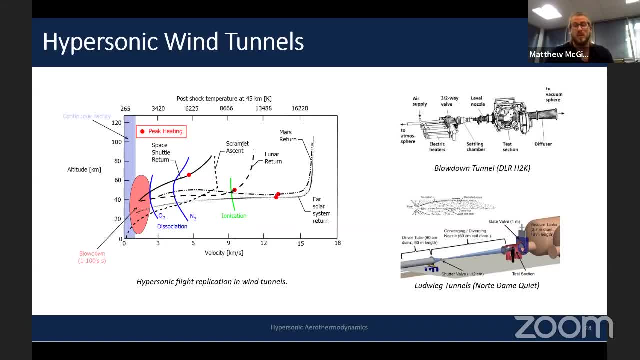 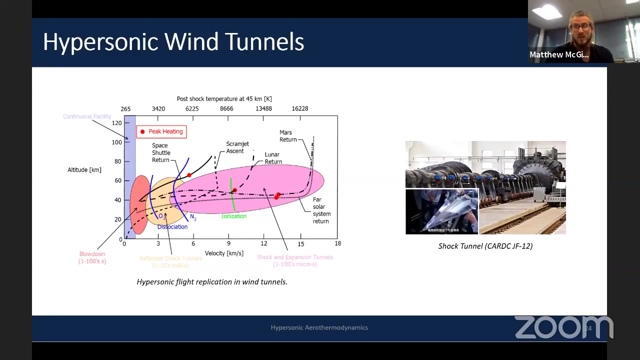 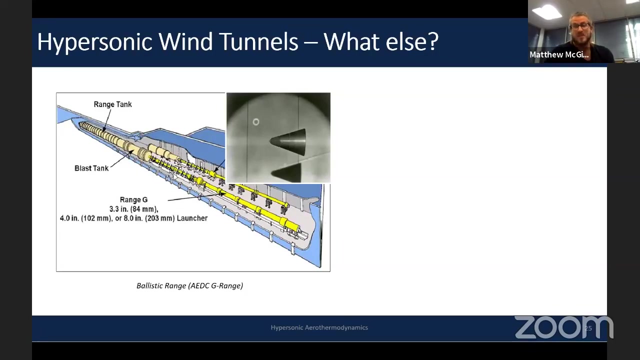 high temperatures um if you've got enough money you know we're talking hundreds of millions if you want to start getting up to 1900 kelvin um but that's only you're starting to tickle where you're getting oxygen dissociation so the only facilities that really can get us up to those super high enthalpies are shock tunnels and then you're only getting test times on the order of milliseconds to microseconds um and you've got to find out where you're going you have to use your own energy from the air huh or you're starting to have a high temperature where you're getting oxygen dissociation you're taking half a day to set up an experiment. The largest one of these in the world is over 300 meters long. I think it weighs over a megaton of steel and they produce a swimming pool full of water at the end. They use a hydrogen oxygen detonation driver to drive the whole processes and it eventually creates water and that then has to be pumped back out at the end of the test. But you know we still can't match everything in that shock tunnels and we don't have enough test time for everything so the next scale up of what could we do for an experiment is you can go have a ballistic range and there's a few of them around the world. 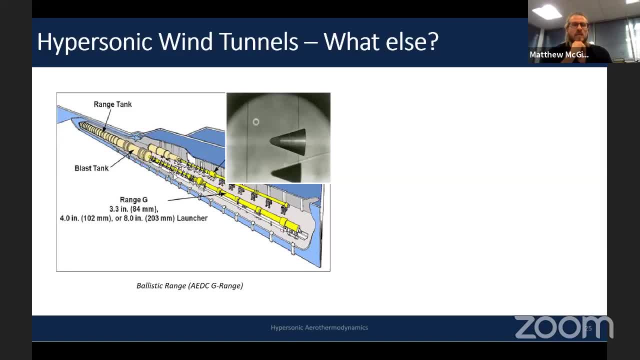 They actually are rarely operated. I was lucky enough to visit G range over at ADC it's a crazy bonkers facility. It's a kilometer long underground. It uses a detonation behind a piston to drive then a compression process of a projectile that's then flung out through a vacuum chamber and it just you measure its flight and any of the other characteristics you want as it free flies down the tunnel for a kilometer and then passes through you know a good couple of you know hundred millimeter steel plates at the end to capture it. 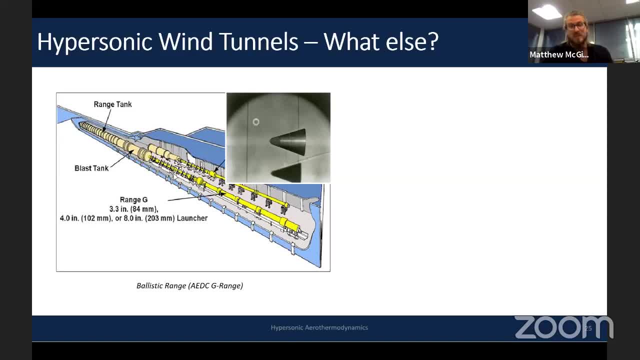 But again you're still dealing with you know teeny tiny hundred millimeter models but at least you're free flying and you can start looking at stability and you know you've got clean air you don't have to worry about that. 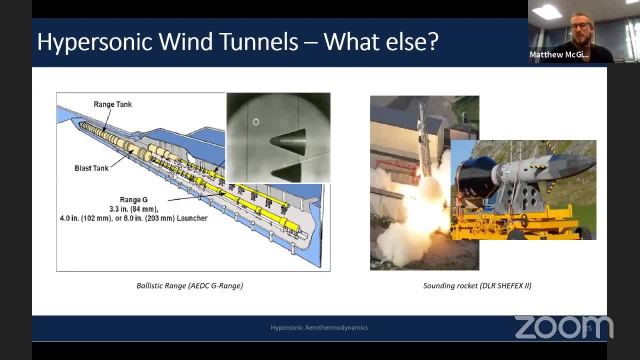 But the real deal is you want to go fly and so you know that that's where you can get clean air clean geometries but to run an experiment on a sounding rocket we're talking about 50 million pounds per per test and at least what I've seen in hypersonic flight 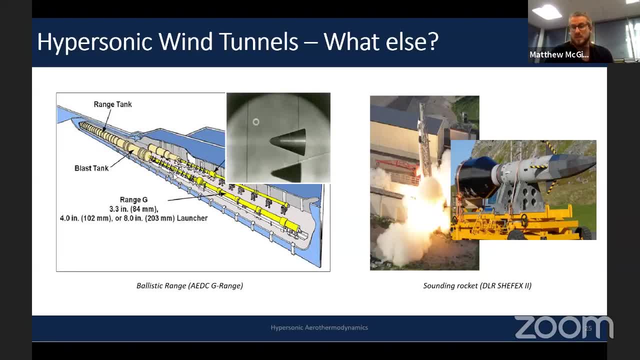 experiments your chance of actually succeeding is about 30 percent. So you want to build three of those to make sure you do get it right so you're talking 150 million pounds to go 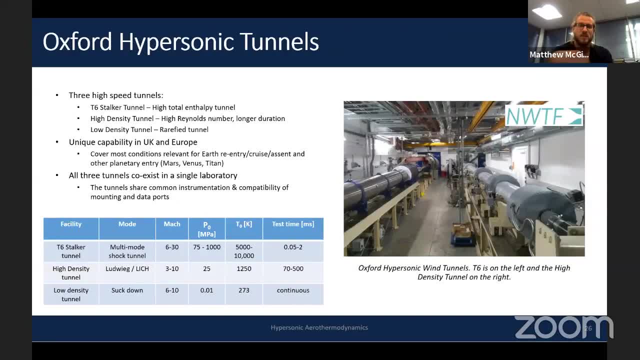 go fly one of these hypersonic experiments. So what we've done here in Oxford over the last six or seven years is to develop really three different high-speed wind tunnels. I'm going to 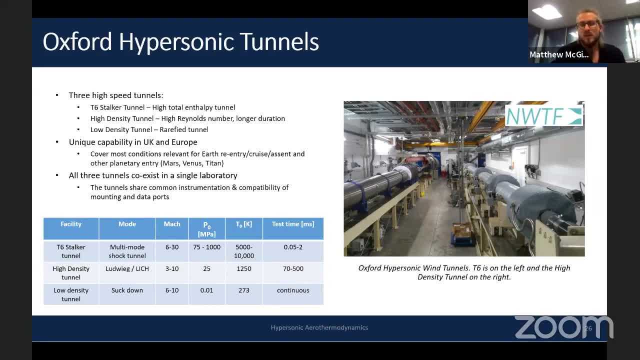 focus really on the first two. So the first is the T6 stalker tunnel and that can match all that thermochemistry which I was talking about earlier but it's limited in test time 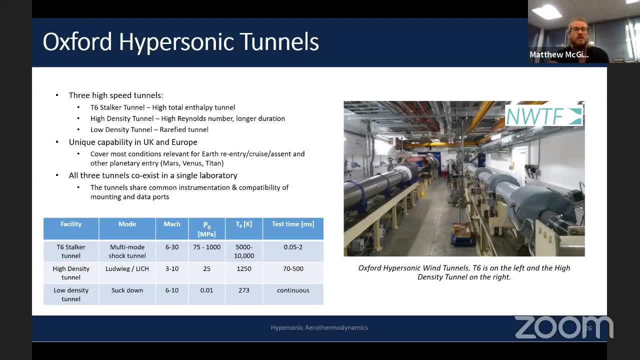 down to the kind of microsecond to millisecond range. So when we want to do longer duration testing, or maybe higher Reynolds number or high pressure testing to match some some of the lower altitude conditions and lower Mach number conditions, we can move across to the tunnel on the right there, 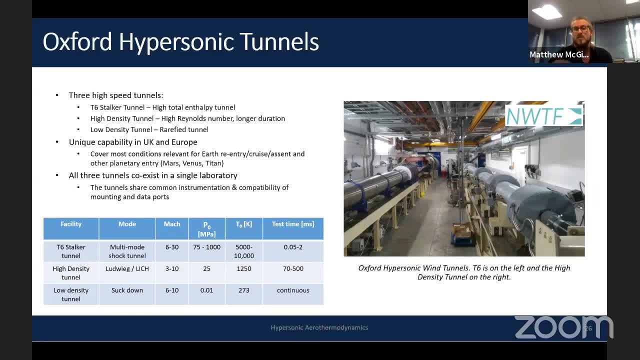 the high intensity tunnel. And so you're really trading off your speed capability, the time capability, but it's all quite nice because both tunnels are sat in the one lab and we can test models in both tunnels, we can test models in both tunnels. So we share a lot of the equipment 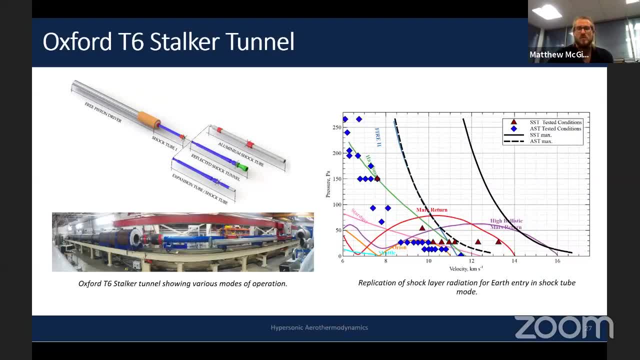 between the two. So to take you through a little just a taster of what these tunnels do, 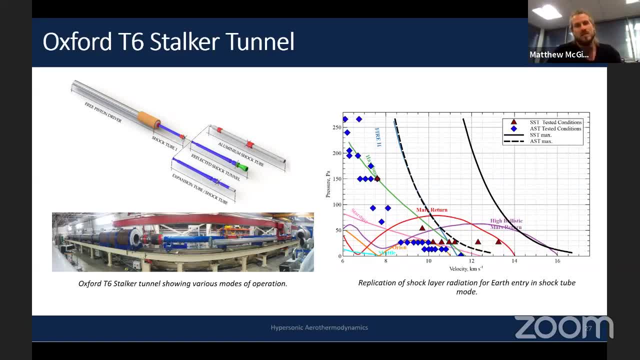 the T6 tunnel is a free piston driven facility. So it has a either a 30 kilo or a 90 kilogram piston that gets flung down the tunnel and it gets up to about 300 400 meters a second. So you can see it travels about five meters and then decelerates very rapidly pulling 10,000 g. So the big mild steel part on the left is really just inertial damping weight because the stress waves become too high for us to handle in an engineering perspective. And once that that gas in the driver is compressed to high enough pressures, it will rupture us a steel plate, which could be a couple millimeters thick. And that high-pressure, high-temperature drive gas wants to then shovel the lower-pressure test gas down to the right, and it will use mechanisms like shock waves to heat that gas up. We then feed it out onto models, typically, but as I showed you earlier, it could be a shock tube experiment where we just take an image as the shock flies past. 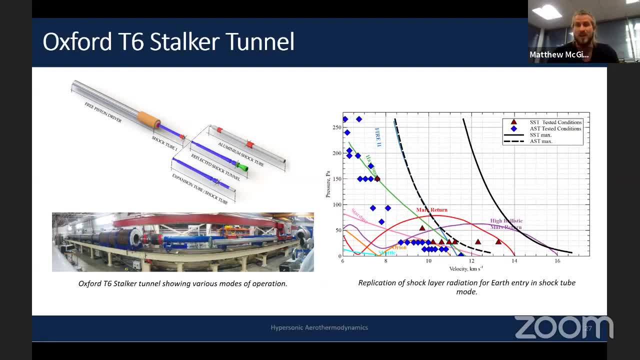 And so you can see on the right, these are really the shots we've been doing over the last six months in blue. And you can see we've kind of spread ourselves around in looking at different conditions from high ABUSA return all the way back to some of the Mars return conditions. 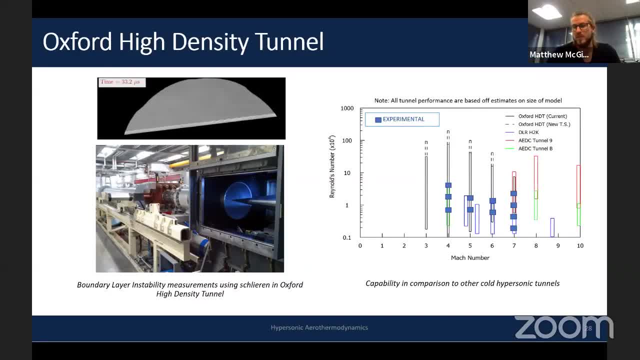 So the high-density tunnel is a Ludwig tunnel. So essentially, it operates by having a big high-pressure reservoir at reasonable temperatures, a couple hundred degrees C. And then we have a fast-acting valve, which is just behind that red gate valve, and it flows through a converging-diverging nozzle onto a model. And so this experiment here was measuring boundary layer instabilities. So we had five megahertz Schlieren running, which measures the density gradients in the flow. And you can see those little kind of rope-like features build up, and they're the precursor. And then you can see the turbulence box growth, and then eventually turbulence downstream. 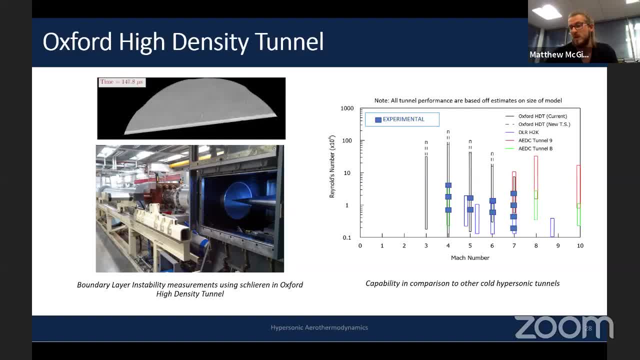 So it's can we understand those processes of boundary layer instabilities, which then eventually lead to transition. 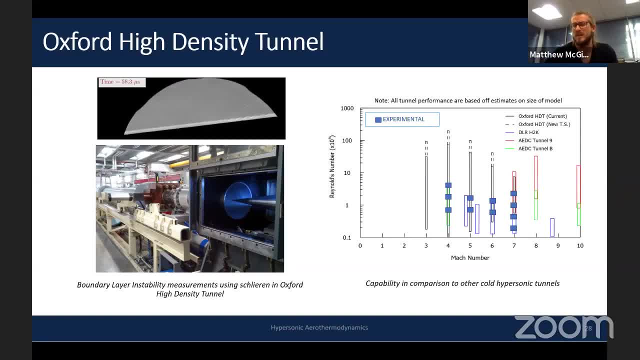 And so you can see where our tunnel sits in comparison to some of the other big tunnels around the world. And when I say big, I mean big. They're kind of, you know, you can fit two humans standing on each other's, with one standing on each other's shoulders in these tunnels. They're very big. 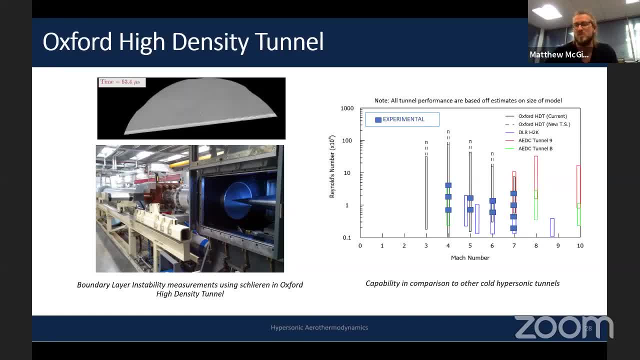 The difference with our tunnel is we can go to very, very high field pressures, which allows us more Reynolds number capability. 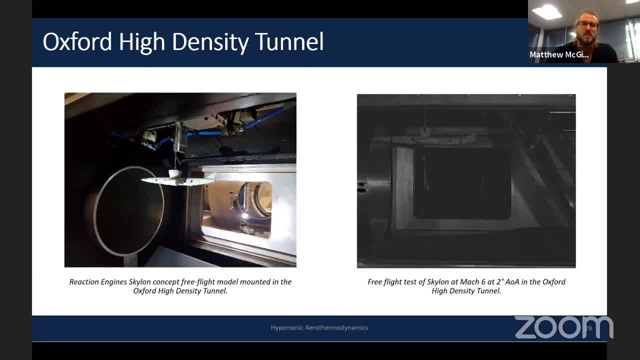 I didn't have enough time in this talk to really talk about aerodynamics much, but I thought it's a really cool video, so why not show it? So this was a test done by one of our fourth years, who's now a DECL student, a few years ago, 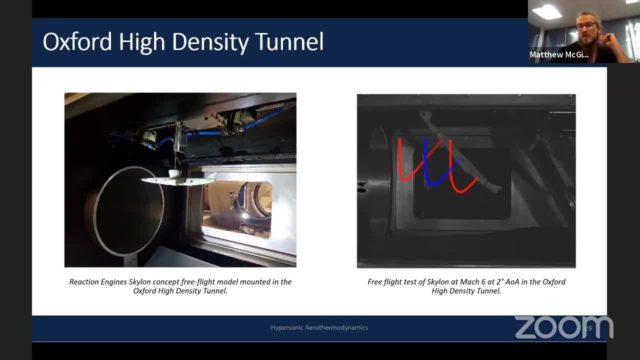 where we free-fly some of our models in the test. 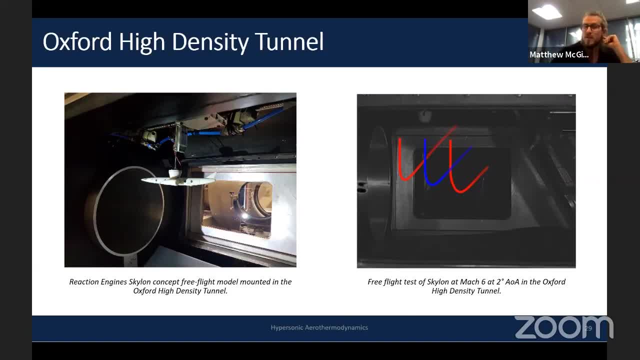 So this is a test section, and we image them at high speeds, and from tracking them, we can then back out the aerodynamic coefficients of forces and moments. And you can see here that this space plane isn't very statically stable, because it just picks up and doesn't really fly where you'd want it to. Instead of flying straight backwards, it flies up very, very rapidly. 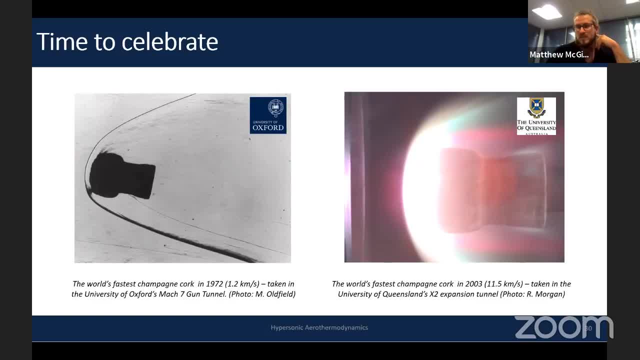 So, thank you very much for having me speak today, and I'd be happy to take any questions. Okay. 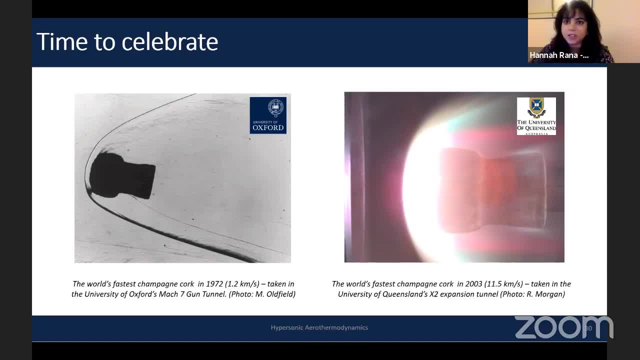 Great, thank you so much, Professor McGillivray. If you'd like to stop sharing, I can... 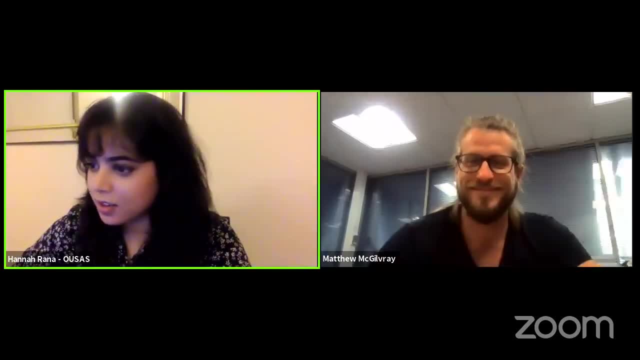 I've got a couple questions. We've got a couple of questions here coming in. 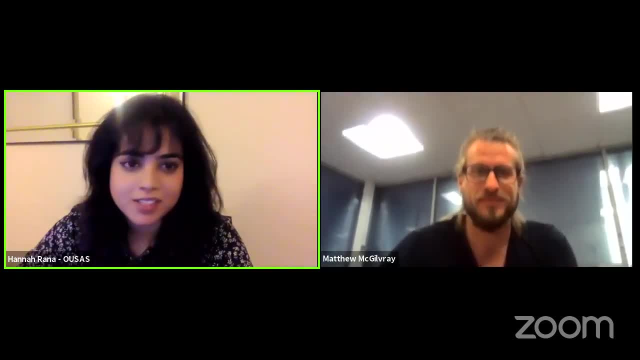 Thank you so much for that very comprehensive talk. It's really fascinating to see a lot of the videos and images you included as well. 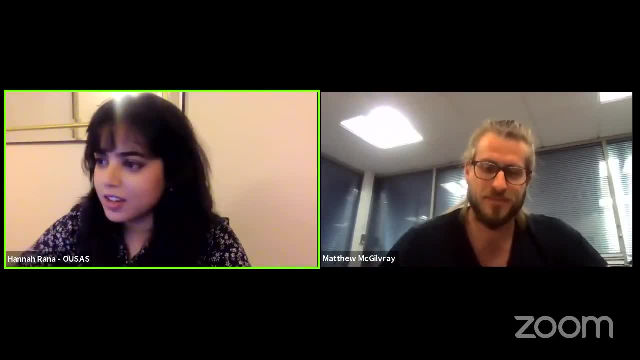 Quite an impressive facility that you're running. 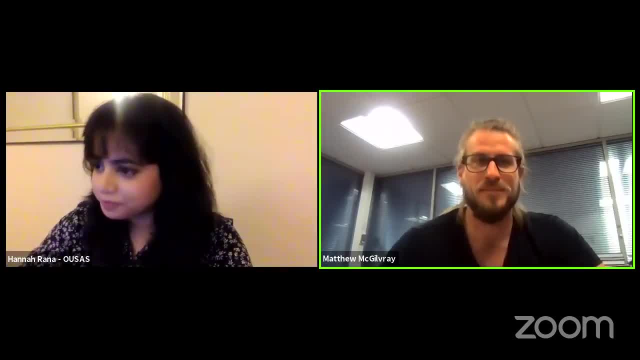 So I'm going to jump right in, if that's okay. Yeah, no, go ahead. One question, which is, in a hypersonic craft, how would the internal temperature be moderated so that internal components aren't superheated? Presumably, there is a great deal of absorption. A really good question, and insightful as well. So, hypersonic vehicles, it depends on the vehicle, actually. 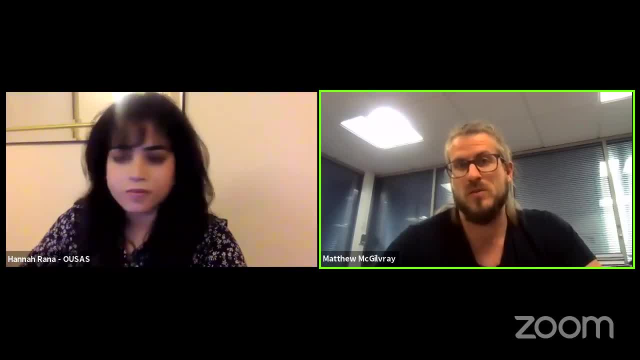 So, some will try and run a cold structure, so you ensure that your heat shield on the front never has any heat soakage into the vehicle, because you can use radiative shields between that very hot object at the front and your substructure. But once you get up to enough flight duration, you're going to get it in there. So that works for kind of shorter duration flights. So, you know, reentry-type flights, that might work. 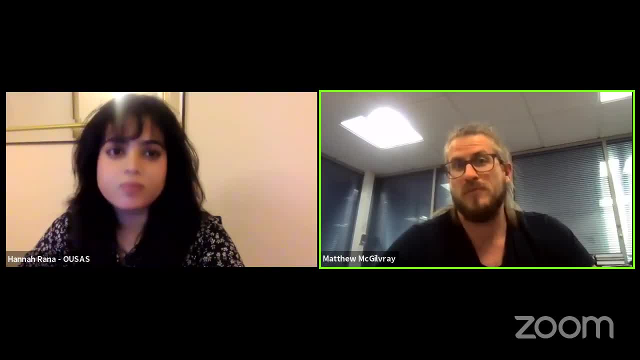 But if you're doing longer cruise, you then have to use hot structures. So you're going to have to deal with the fact that you're hot. So you want to actually get some of that heat away to the back of the vehicle where it might be cooler for it to just re-radiate out. So it's a game of, well, you're going to have to... You're going to have to design for having hot bits in there. But it's all about, can you get the conduction pass to where you can re-radiate it out back into space and convect, if you can get the flow cold enough again. Okay, great. Thank you so much. So there's another question. What are the benefits of using active cooling over opting for ablative technology? 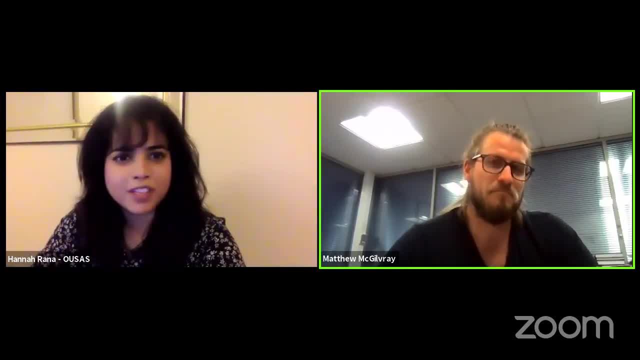 Yeah, I think I actually... More effective is one over the other. It's hard to beat ablators, just as an honest opinion of someone who's researching transpiration cooling and active cooling. Ablators are very lightweight for the amount of cooling they can give you. 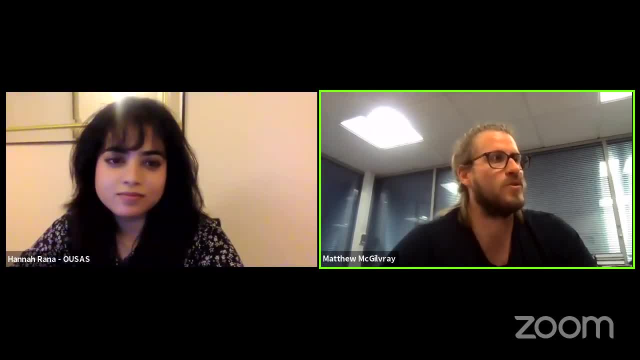 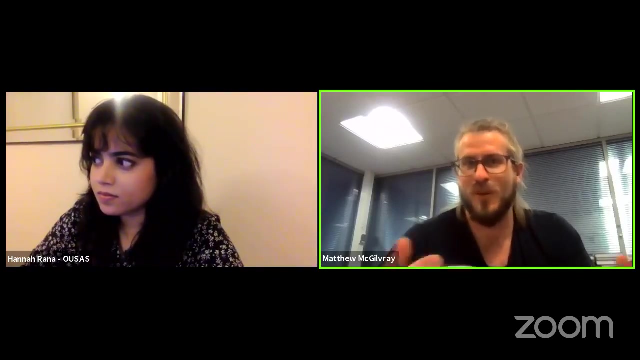 Extremely lightweight. Now, the two bits is if you have it for a sharp bleeding edge, there's an obvious thing that with an ablator, you're trying to have a sharp bleeding edge for aerodynamic efficiency. So you want it as sharp as possible. We're talking down to the millimeter scales. And if you have an ablator, you'll very soon not have a very sharp bleeding edge. So you've kind of lost the game of why you wanted to have a sharp bleeding edge. So that's why we're investigating this technology for it. The second... 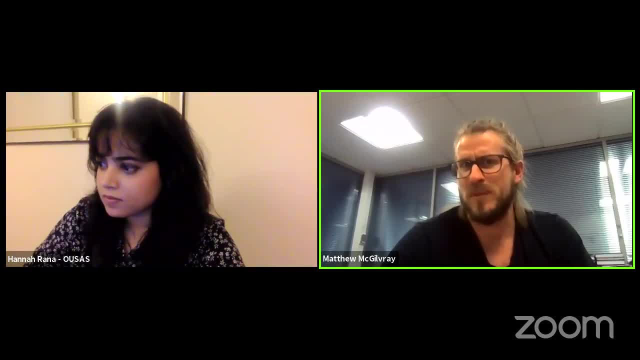 Well, there's quite a few more in terms of military applications. So it could be observability. 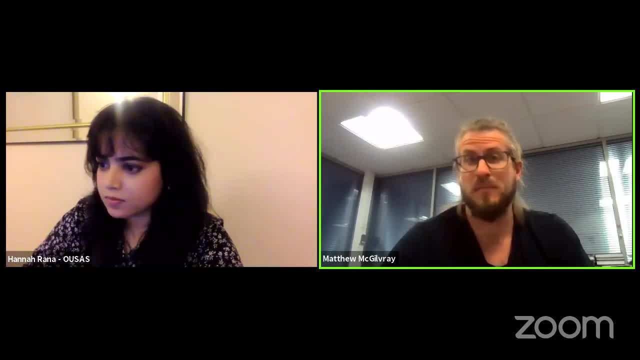 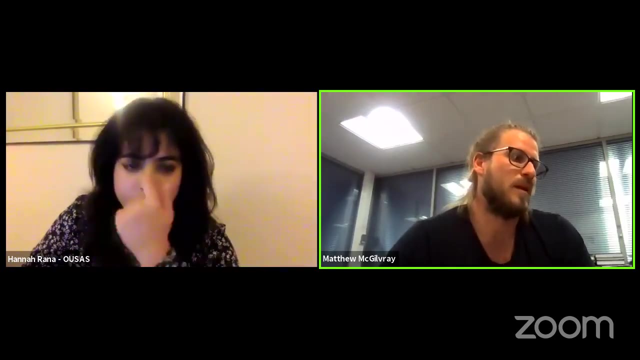 Carbon coming off an ablator is very, very pronounced. It radiates like all hell. It could be also protection of IR windows and sensor windows where you actually want to see out of them. So having an ablator come past with a lot of carbon is a bit of an issue. But what you pay for with any active cooling system is the complexity budget. Even if the mass is comparable, which it probably won't be, ablator will be lighter, the complexity goes up enormously. 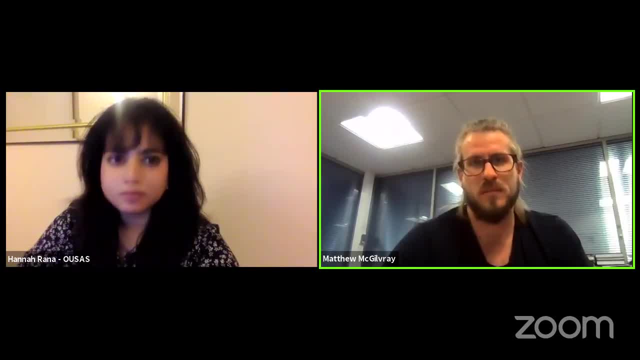 So you really would want to... You have to have good reasons to go to it. You would choose if... Everyone will choose an ablator every day of the week, unless you've got very specific needs. 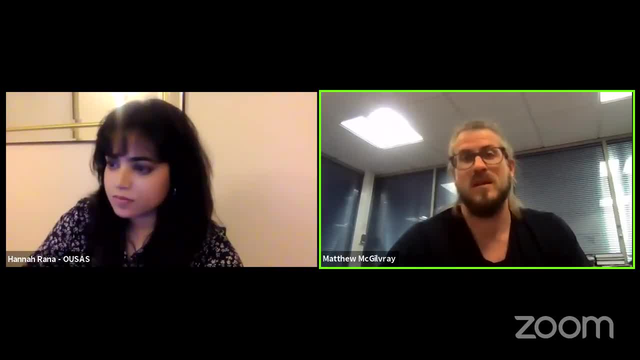 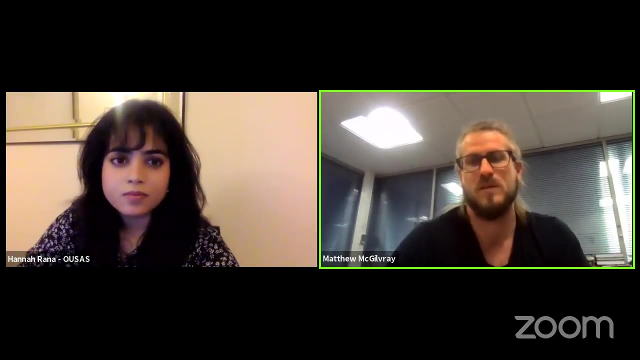 And reusability is probably one of the highest. That if you want to have a space plane that flies continuously, if you have an ablator, you've got to change it every time. When the spacecraft lands, you've got to strip the whole thing off, put on a new ablator. And that obviously leads to higher risk that something's going to go wrong. 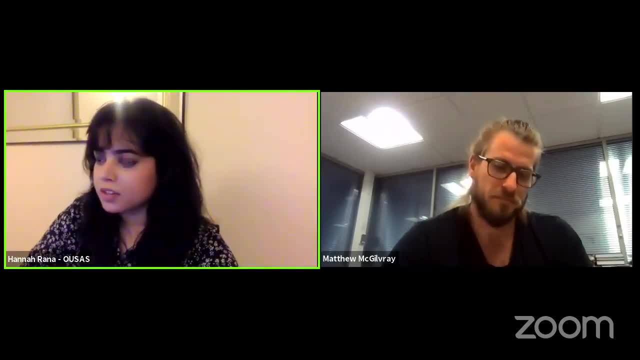 Have you worked on dynamic or moving models, for example, deployable structures? And what challenges do you face when working with models like these in hypersonic testing than models that stay the same size and form? Good question. 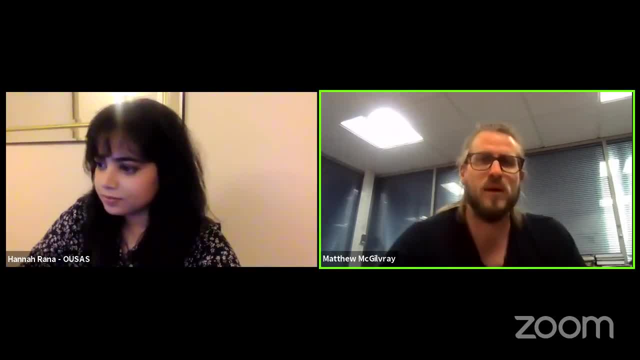 No, I haven't. It is something that we've talked around multiple times. 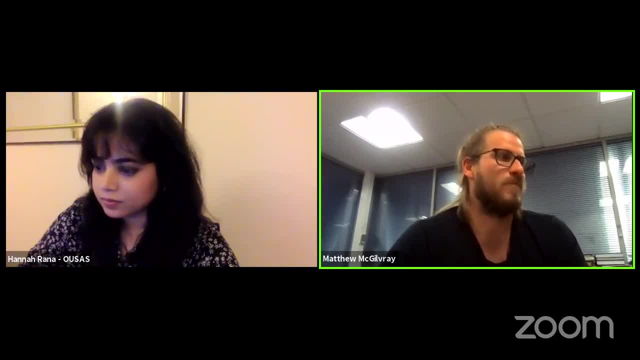 Never actually done. Very, very challenging. 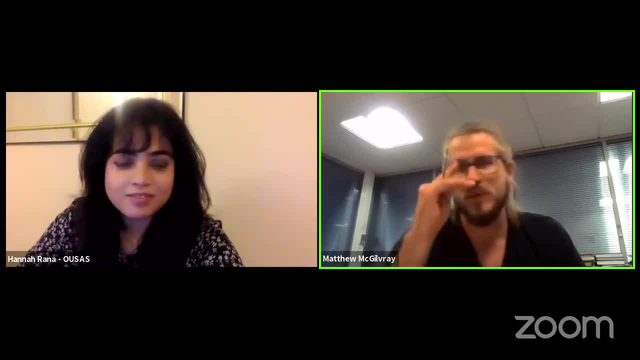 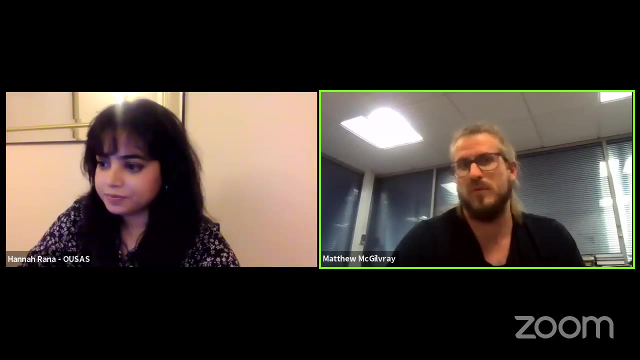 To have moving bits within a test. We have a couple of details that are just starting to look at control systems. So starting with flaps and other parts and looking at control of these things. But deployables is another level of complexity. Because your control of those will be difficult. 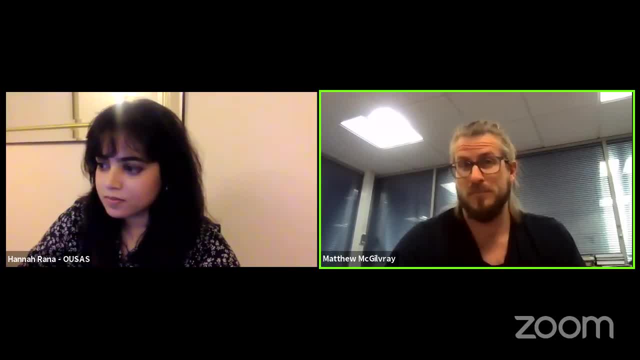 People have done them in these sort of facilities. But they are a difficult experiment. Okay. 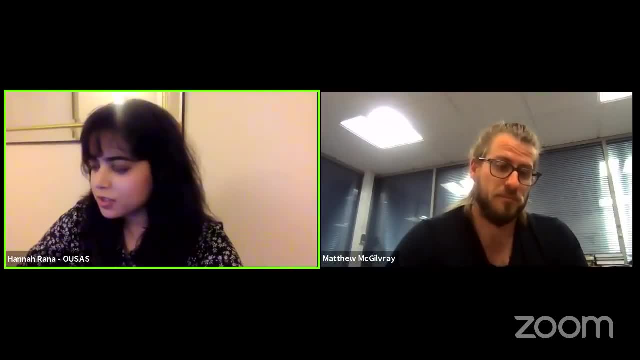 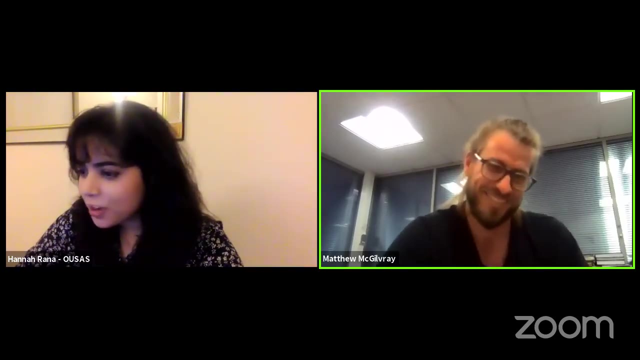 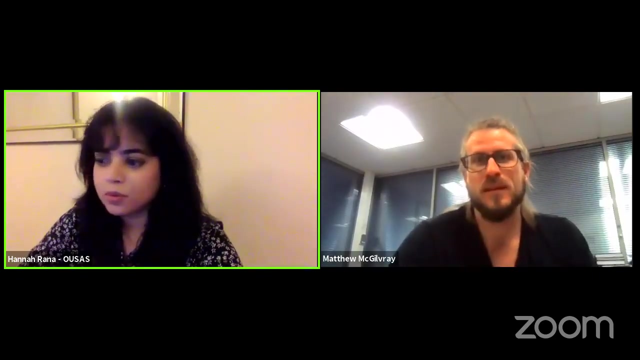 Why not use internal conduction lasers to shoot down the ionization layer to lower temperature to a more operable range? It can be coupled with the active heating system. Might have to ask for that one again, if that's okay. Why not use internal conduction lasers to shoot down the ionization layer to lower temperature to a more operable range? Okay. So. 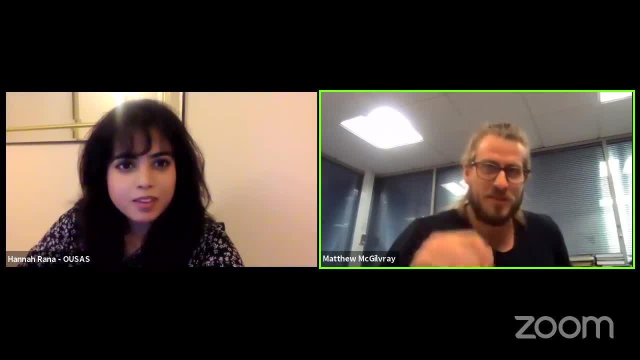 I'm not quite sure I know what that sort of laser is. So I'll just preface it at the start. 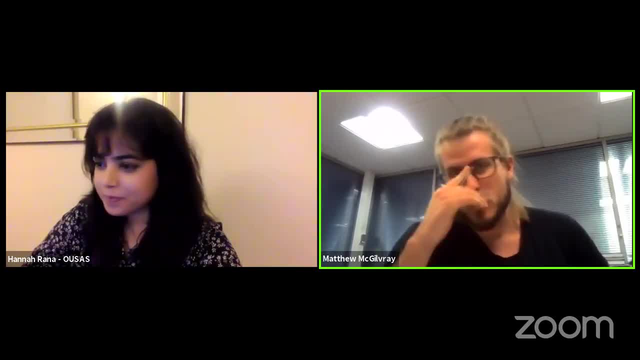 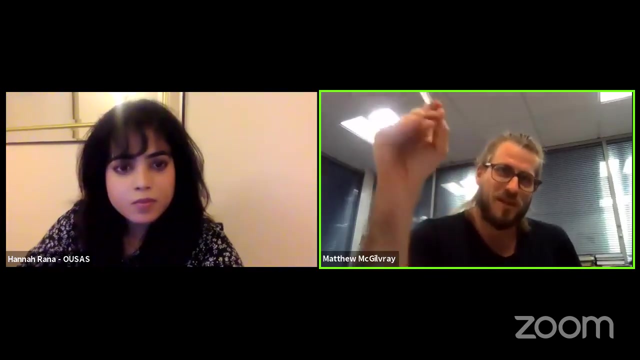 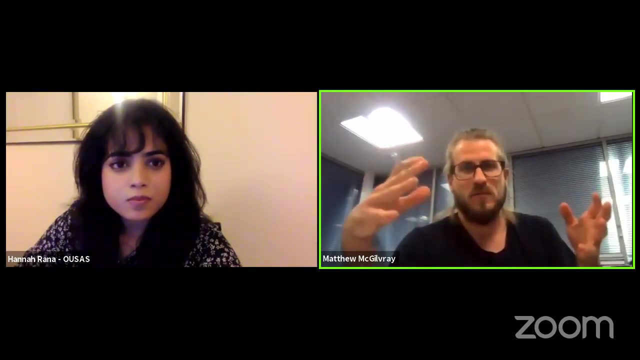 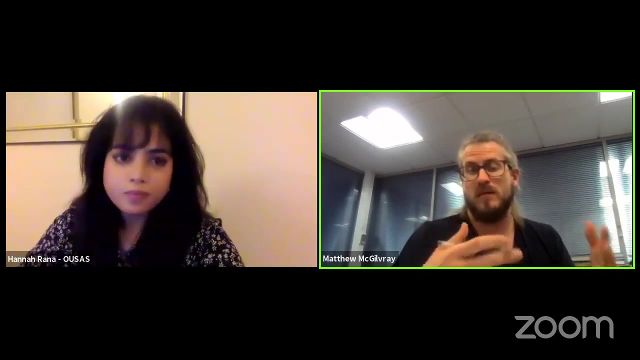 But maybe I can talk about certain things which are interesting around that thought. So one of the interesting things that you could do and people have thought about is actually having a laser and focusing it in front of a vehicle. And essentially mimicking what an aerospike does. So an aerospike is a little object that you can put out the front of your vehicle, which means that the shock to your vehicle, it looks like you've got a, the shock's not sitting right in front of you. You've got something to break it in front of you. And what that can do is reduce drag because your shock's not as blunt. You've actually got, you recover more pressure back on the vehicle. So that's kind of a neat thing that people use lasers for. Now, people have thought about all kinds of crazy, you know, magneto hydrodynamic effects and lasers like that. But anyone that does a simple calculation and sees how much power you need for these things and how big the lasers are and how much they weigh start scratching their heads pretty quickly that, you know, you're 10 times to 100 times the weight of your vehicle very quickly. Okay. There are people that are interested in. For example. For cooling reasons using these strange materials that can, when they get up to high temperatures that they can pass out free electrons. And actually, you're giving off energy by giving off these electrons so you're getting rid of some of the heat through just generating them but you've got to collect those electrons back or otherwise you're going to get a deficit pretty soon and stop the process. But in terms of. 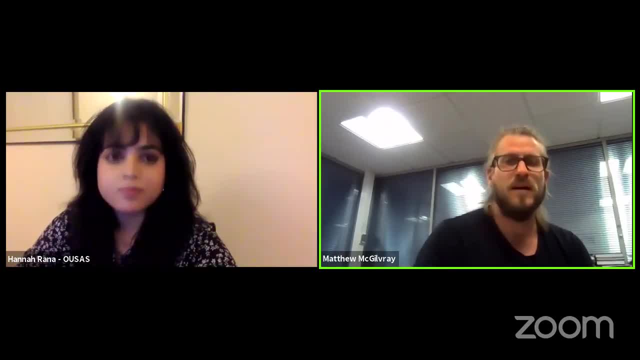 Yeah. I mean, I don't think it's the same technologies that people are exploring, but I tend to find them. Unless there's a huge game changer in terms of mass weight space, it's we're talking hundreds of years away for those technologies to ever come online. Wow. 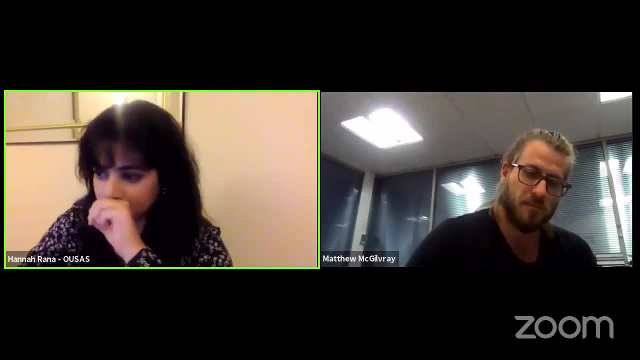 I'm sort of along the vein you mentioned like me too so it says, there's one question if you have dissociation of molecules can use a magnetic field to force the plasma away from the surface. surface. 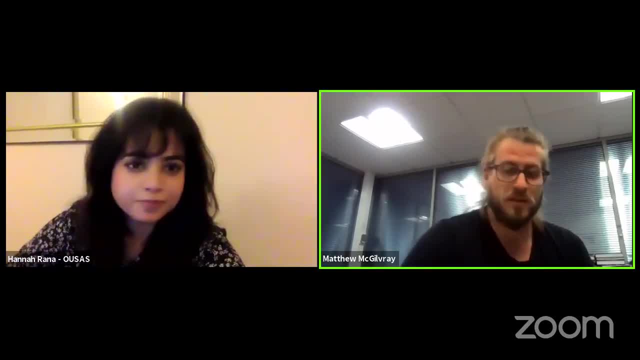 The answer is yes. Yeah. And, and people do look at that very directly. So really good thought and people are researching it. I think it's just the practicality of mass. 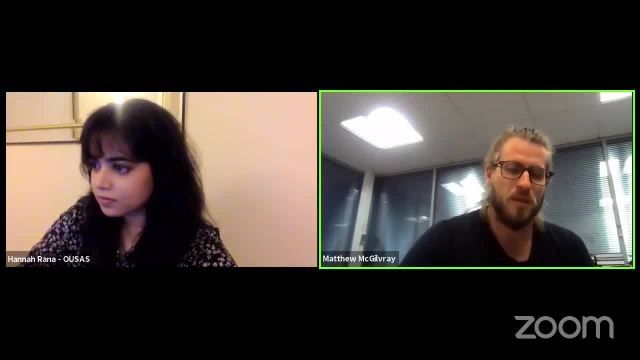 That's the killer for that system rather than the actual physics and, you know, understanding the physics and knowing how to control it in a nice way. People have shown initial results that were actually quite promising. I think it's just that the technology build of those systems is more the, you know, the difficulty and again, complexity, you know, just anything that adds complexity to a spacecraft you want to remove because, you know, the risks are very high that you're going to lose it. 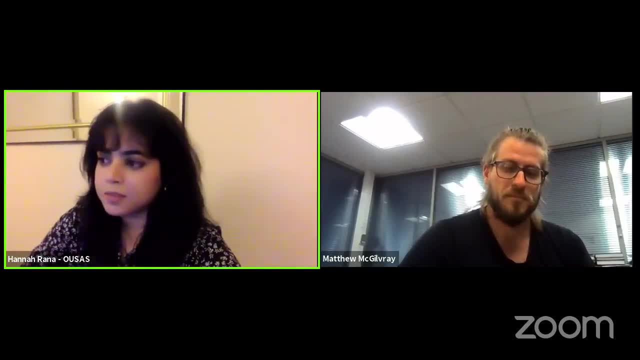 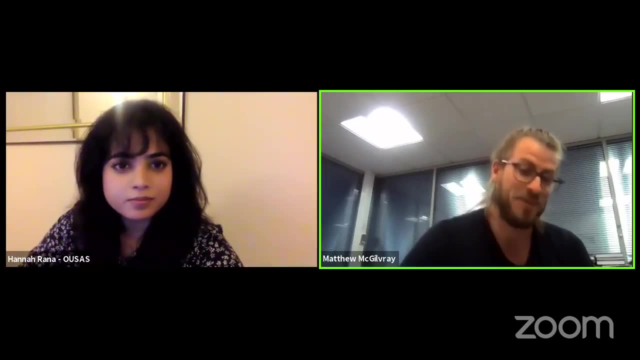 What are the major challenges and differences for Mars missions versus gas giant entry versus ice giant entry? And how do we study these on earth? Good question. 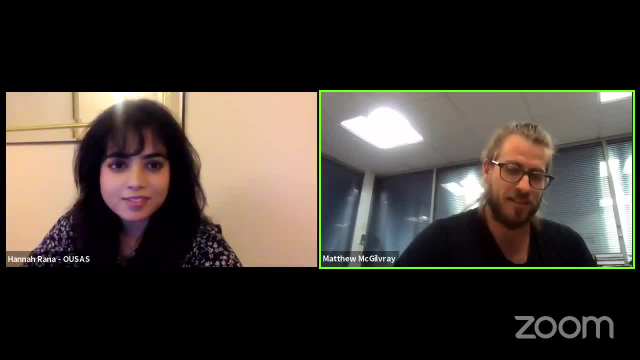 I'm literally going to be called downstairs to, to look at Mars entry in a very little bit. 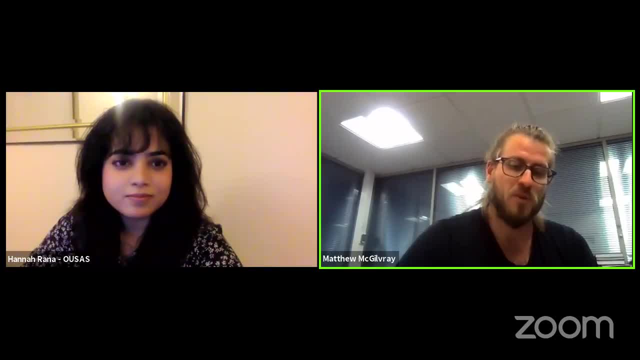 And we've just kicked off a PhD program to look at ice giant entry. So we're very interested in all them. So differences. 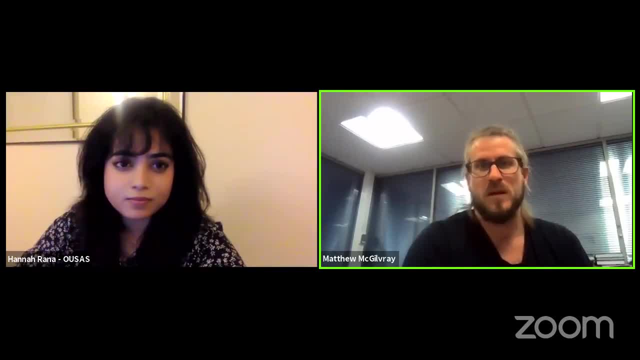 So for Mars is where we're probably going next with humans, right? If we're going to go venture out. 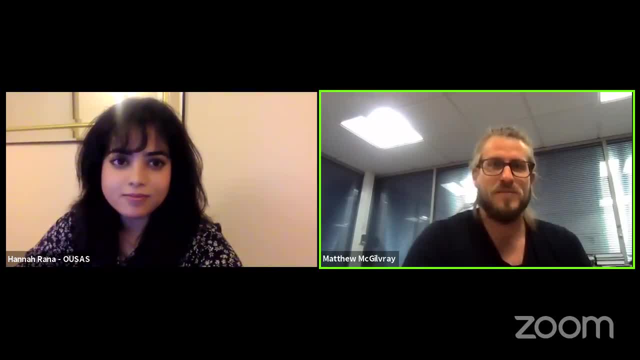 So currently we've landed little robots there that have driven around. That's really cool. But if we want to get humans there, we need lots, much, much bigger vehicle to enter Mars. And that means much bigger shock layers. So the radiative heating back to the vehicle goes up. So from an engineer's perspective, it means that we want to know more about that radiative heating than we ever did. And that's something that we've never had before because it just didn't matter for the smaller probes, but now we're getting bigger and bigger. The amount of gas that's compressed on the front that can then radiate back is increased. 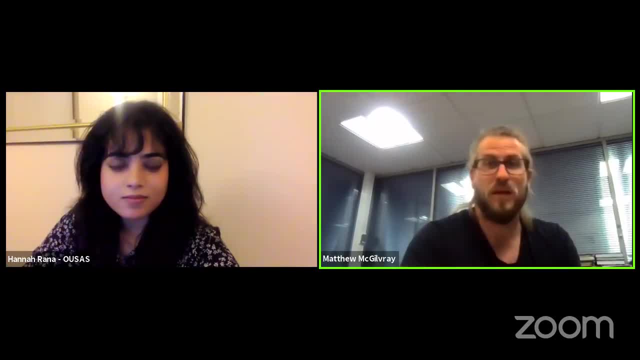 And in particular, there's big uncertainty on, interestingly on the back shell of vehicles. 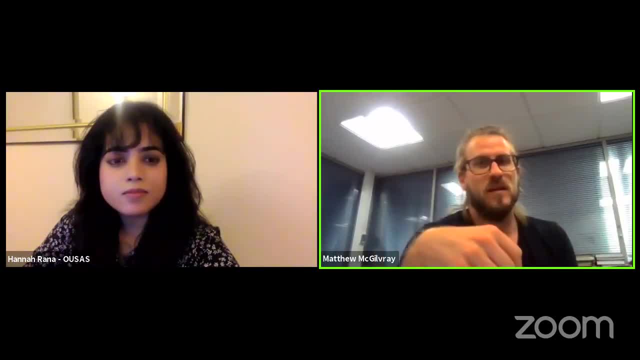 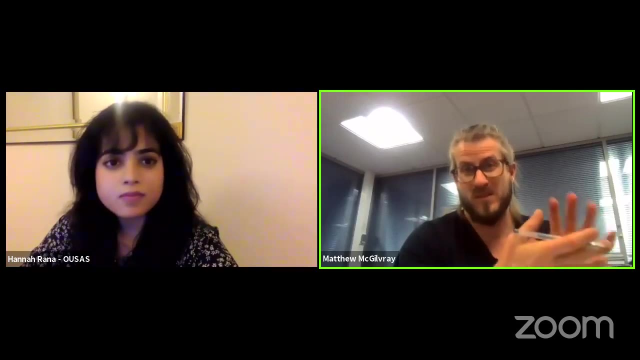 So not where the hot plasma is once it's expanded out, it can, it can actually stay energized for certain vibrational states of, of, of, of STN which radiated in the mid wave in for red and compound back. And so it means that you might actually need, you know, 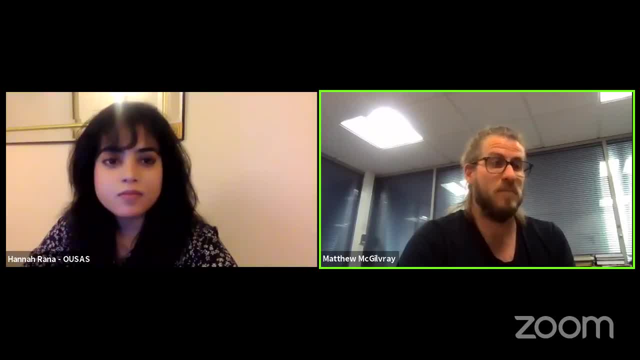 they're predicting quite thick bits of TPS on the back of these vehicles because of the high uncertainty there. 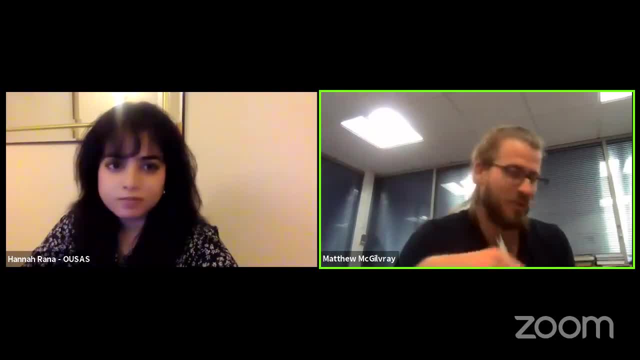 So the major difference is speed and gases, probably as a general statement, speeding, speeding gases. 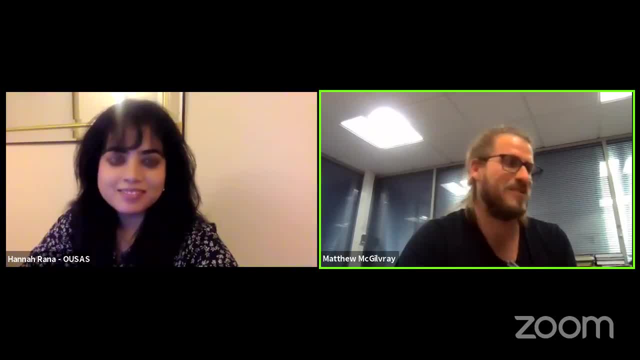 So Mars entry is gentle seven kilometers a second, and it's mostly CO2 with a little bit of Nice. Um, when you go into the ice giant and and it's like, like the weather is not good. So you've got a little bit of nitrogen, 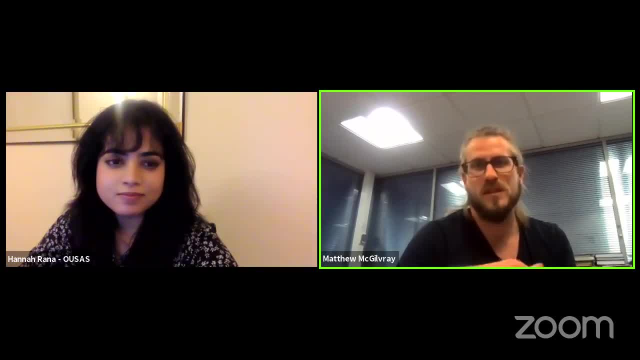 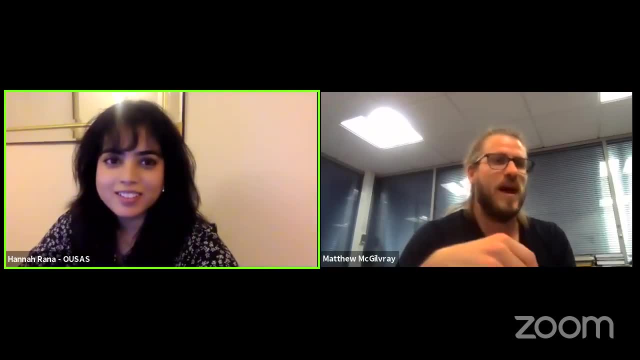 and the gas giants uh you're you're talking hydrogen helium systems and you're talking 20 kilometers a second or above wow um so and radiative heating goes up with about velocity 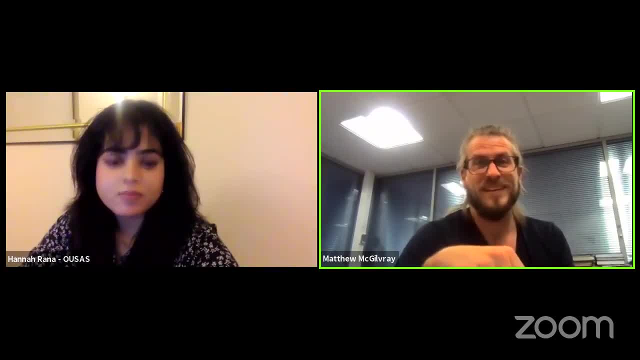 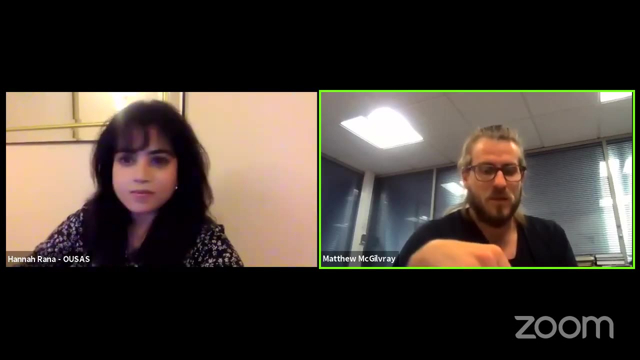 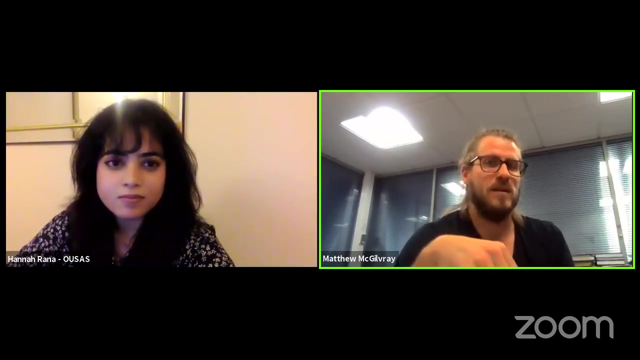 to the power of four i think that's the top of my head uh so the the amount of heating rapidly goes up um due to that uh it's the the amount of radiative heating for hydrogen helium systems isn't as high as you'd expect at 20 kilometers a second because it hangs things don't quite getting as energized as they would but for jupiter it's just all radiation it's huge um we've actually got loads of questions coming but i think in the interest 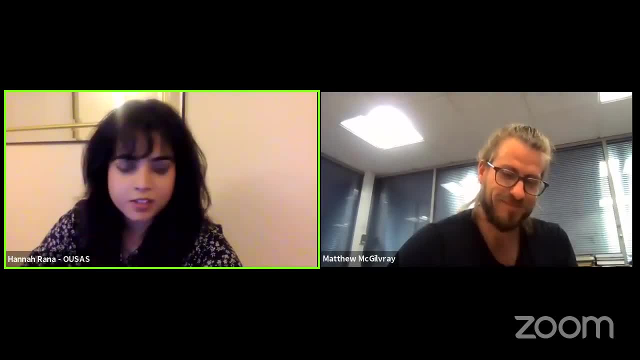 of time um i'll ask one more question and after that a general question that that we tend to ask so what are the next developments in the lab and what is the next big problem progress we made in hypersonics 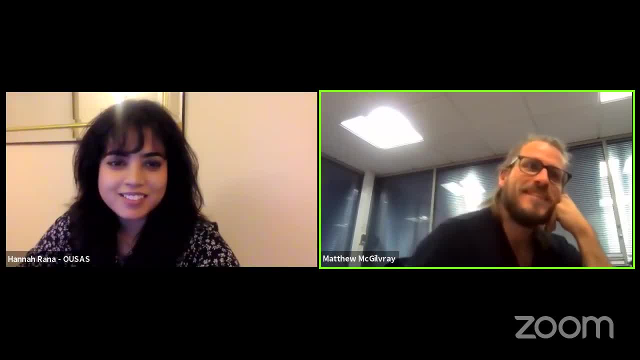 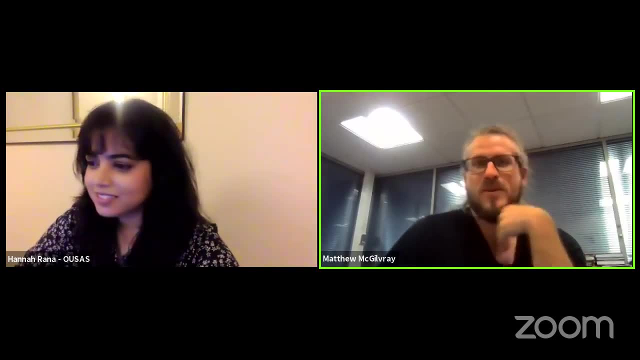 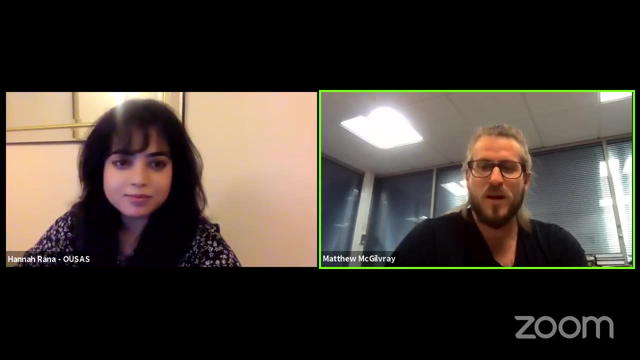 god what's the next progress in the lab um that's a really great question um so at the moment um i think we've got quite we're kind of we've got a lot of students working on transpiration cooling work but i think that's kind of you know we're kind of moved that up a little bit in the trl chain um what what's going on with that um i think probably i would suggest that my 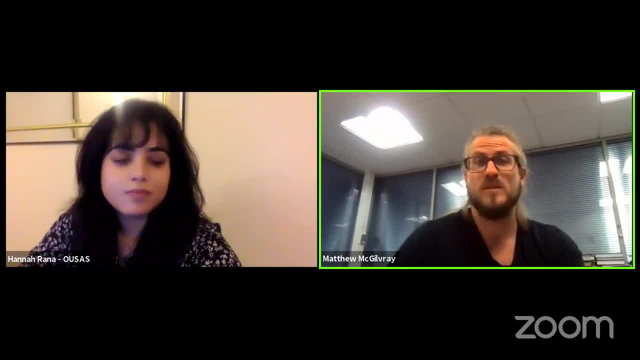 my new colleague uh tobias herman is probably doing the most exciting thing that could happen um in terms of development so he's thinking about combining one of those plasma wind tunnel facilities with our short duration shock tunnel and if you can do that it means you can do hot hot surface temperature or ablative testing coupled with a short duration shock tunnel with the wind tunnel flows so because we have such short durations the models stay cold they'll only rise by a couple of degrees kelvin over our test times but if you could preheat them and get 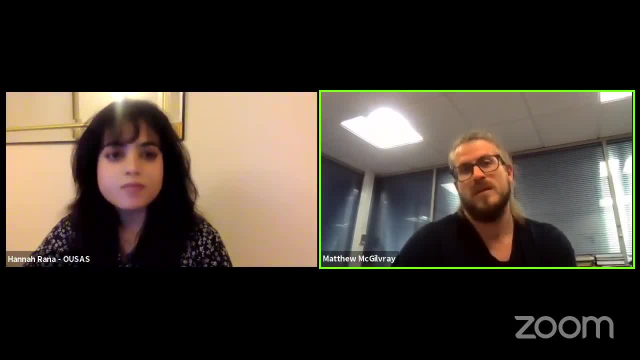 the ablation started and then pass the flow over them you can actually start thinking well okay well uh we might be able to do realistic coupled studies of the aerodynamics and the ablative together um so i'd say that's probably 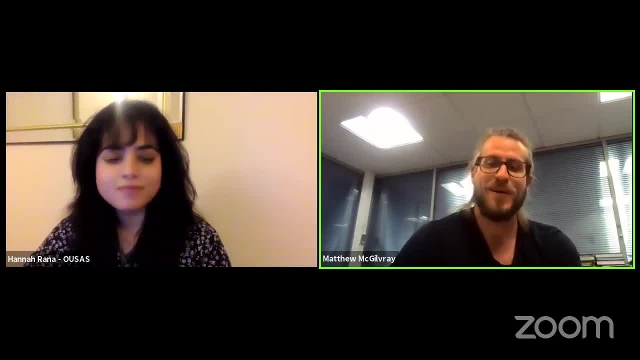 the the most exciting and the the grandest challenge um when it comes to to a i guess the experimental side um in terms of generally what's what's happening um well ice giants is probably the most interesting or titan entry at the moment in terms of if i want to think space 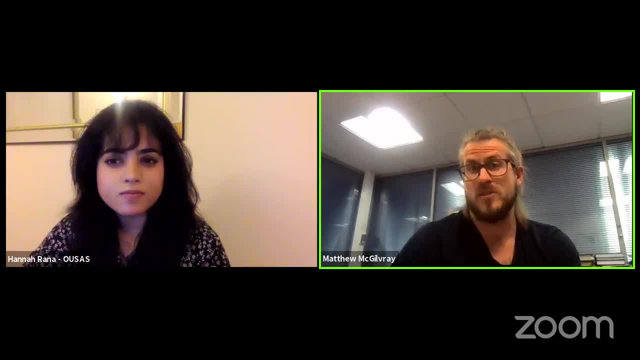 because um there's a there's a window to get to the ice giants and nasa and easter are considering it um going after it as a combined mission 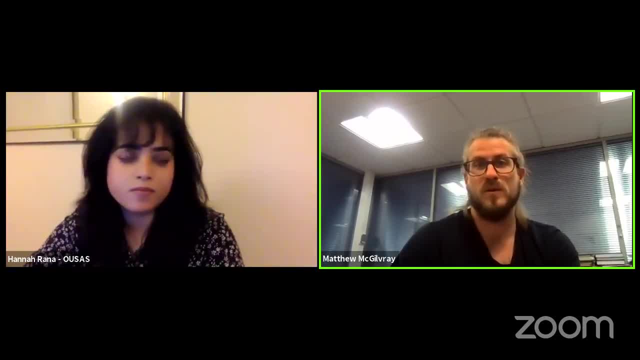 um so we're doing kind of first-phase low low trl studies to see what what the capability is required um for those and titan they're going to go fly a quadcopter so one of my best friends from undergrad is leading the the nasa dragonfly mission so they're going to try and get into 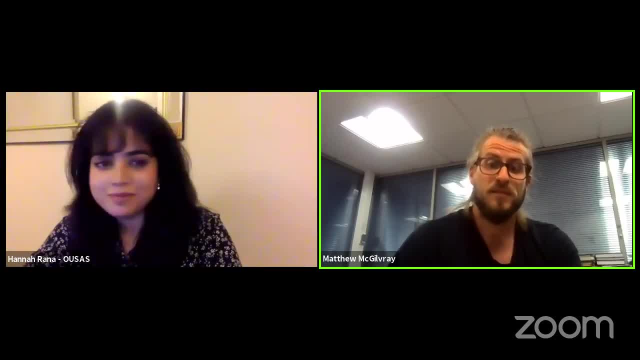 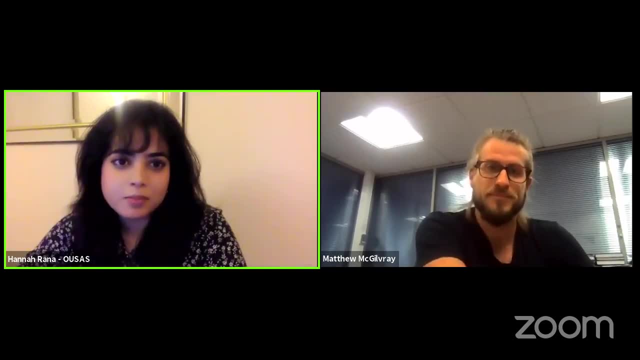 titan and fly a quadcopter around yeah excellent um so last question um something that we ask all of our speakers um what advice would you give to people who are interested in flying a quadcopter 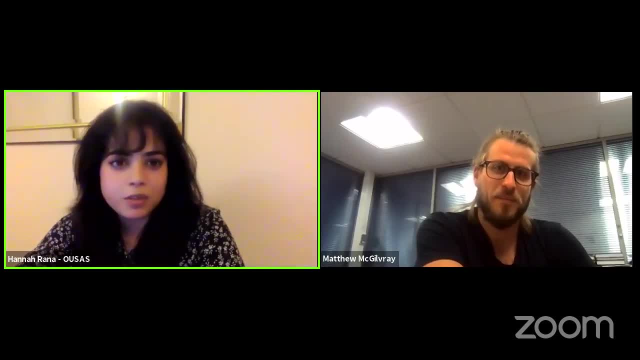 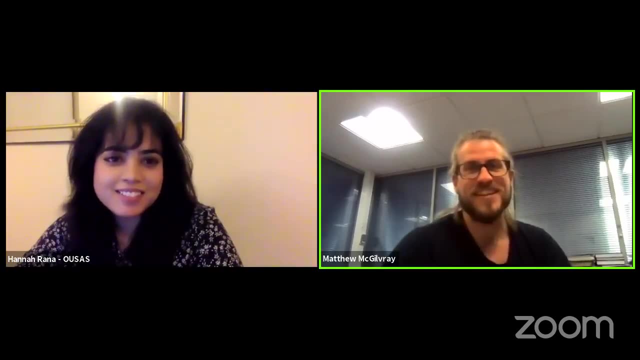 what advice would you give for early career researchers looking to refine their research focus and just any general advice um take a chance see if it was the i i remember i didn't know what